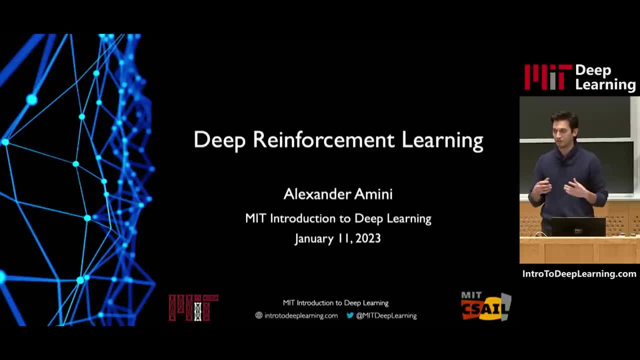 in this lecture right now, I'm going to start to talk about how we can learn about this very long-standing field of how we can specifically marry two topics, The first topic being reinforcement learning, which has existed for many, many decades, together with a lot of the very recent 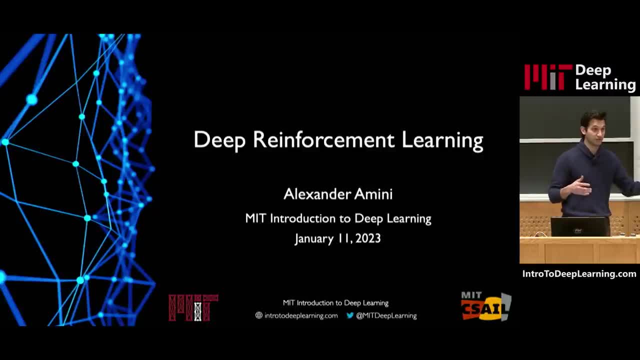 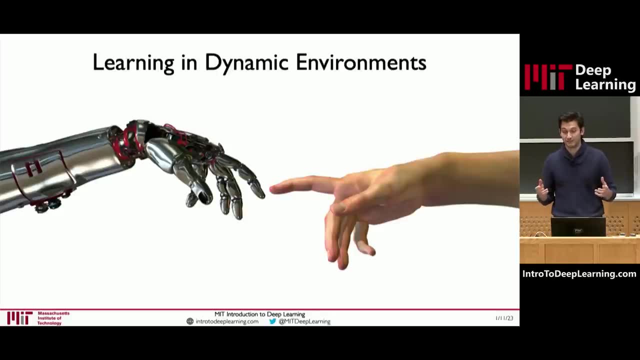 advances in deep learning, which you've already started learning about as part of this course. Now, this marriage of these two fields is actually really fascinating to me, particularly because, like I said, it moves away from this whole paradigm of, or really this whole paradigm. 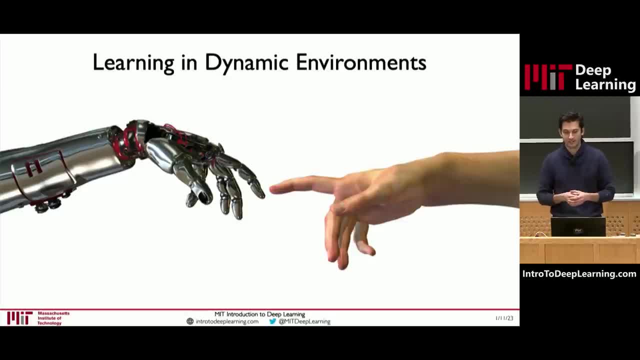 we've been exposed to in the class thus far, And that paradigm is really how we can build a deep learning model using some data set. but that data set is typically fixed in our world right. We go out and collect that data set, we deploy it on our machine learning. 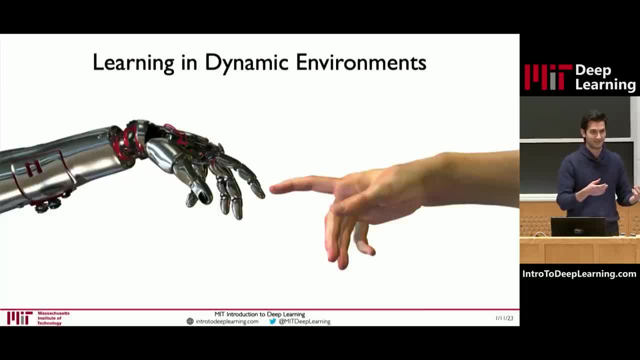 or deep learning algorithm, and then we can evaluate on a brand new data set. But that is very different than the way things work in the real world. In the real world you have your deep learning model actually deployed, together with the data together, out in the 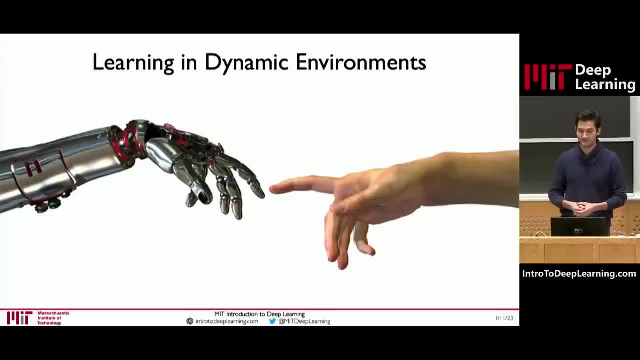 world into reality: exploring, interacting with its environment and trying out a whole bunch of different actions and different things in that environment, in order to be able to learn how to best perform any particular task that it may need to accomplish. And typically, 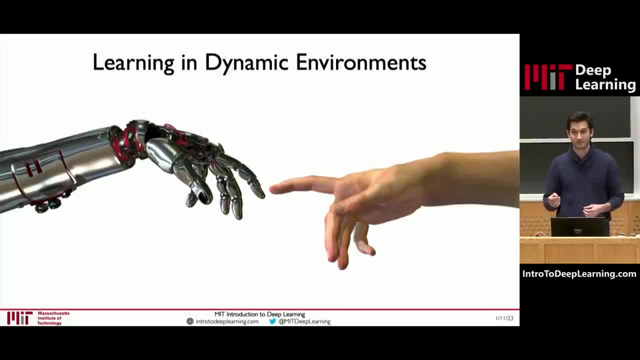 we want to be able to do this without explicit human supervision right. This is the key motivation of reinforcement: learning You're going to try and learn through reinforcement, making mistakes in your world and then collecting data on those mistakes to learn how to improve. 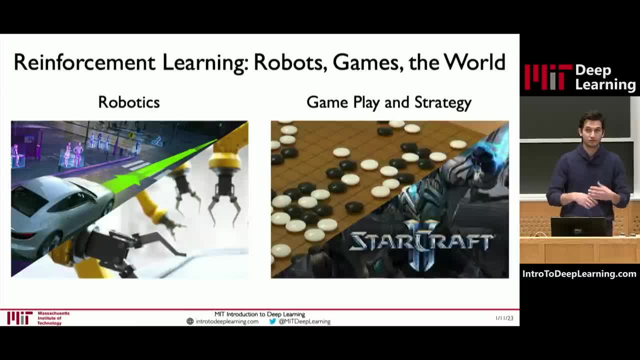 Now, this is obviously a huge field or a huge topic in the field of robotics and autonomy- You can think of self-driving cars and robot manipulation- but also very recently, we've started seeing incredible advances of deep reinforcement learning, specifically also on the side of gameplay and strategy making as well. So one really cool thing is that. 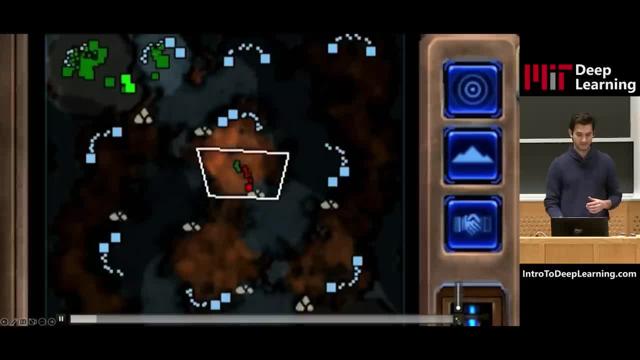 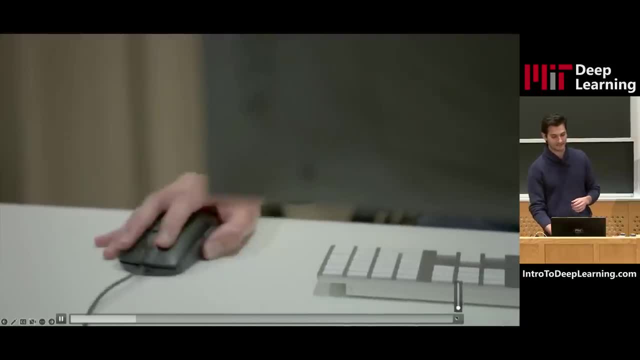 now you can even imagine, right, this combination of robotics and self-driving cars and robot mechanics, together with gameplay right Now, training robots to play against us in the real world. And I'll just play this very short video on StarCraft and DeepMind. 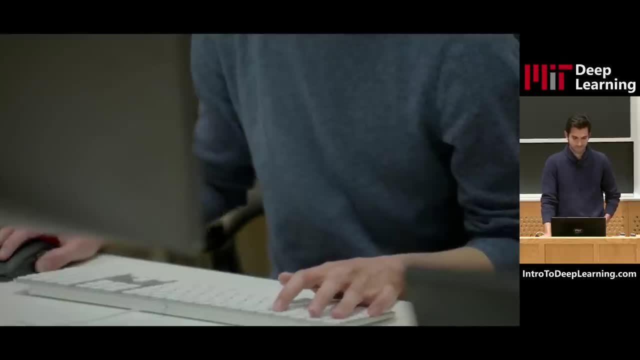 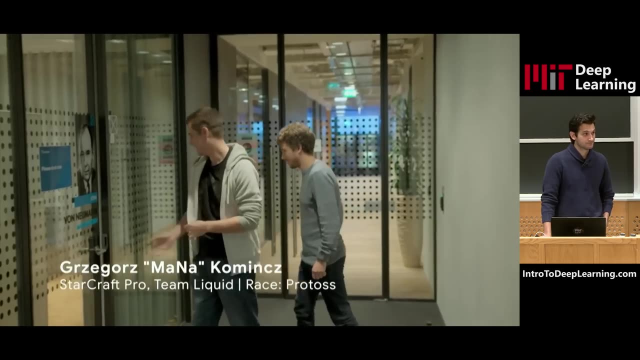 Perfect information and is played in real time. It also requires long-term planning and the ability to choose what action to take from millions and millions of possibilities. I'm hoping for a 5-0, not to lose any games, but I think the realistic goal would be 4-1 in my favor. 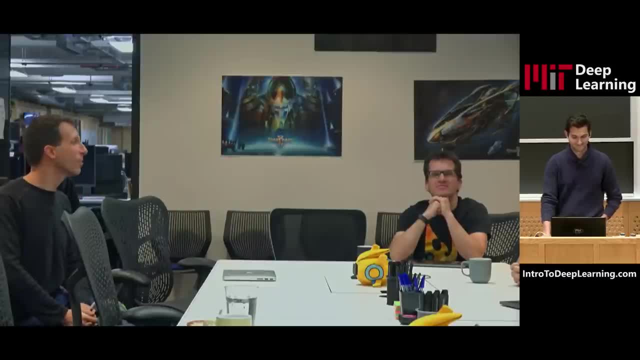 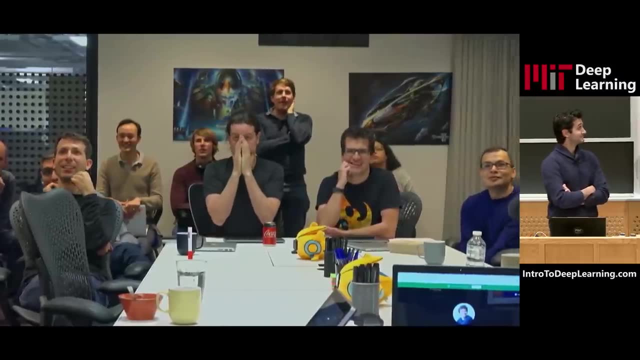 I think he looks more confident than Tiolo. Tiolo was quite nervous before. The room was much more tense this time. Really didn't know what to expect. He's been playing StarCraft 3D. my sense is he's 5.. 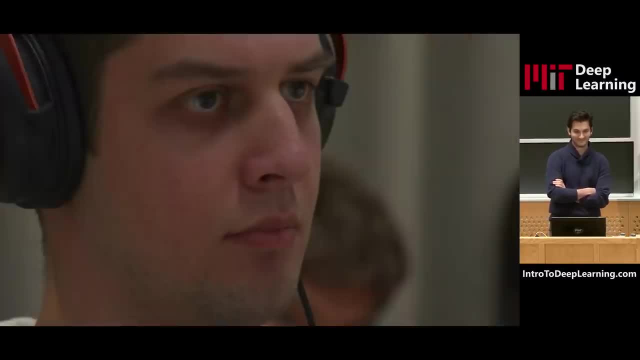 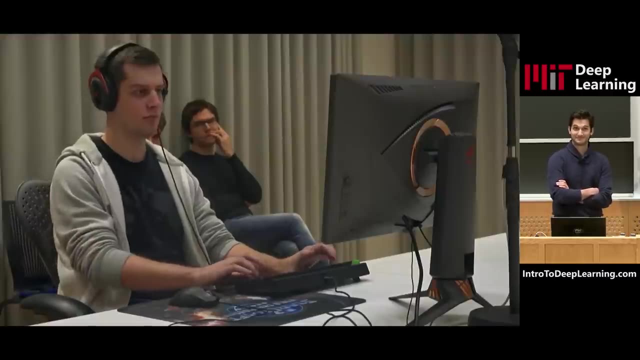 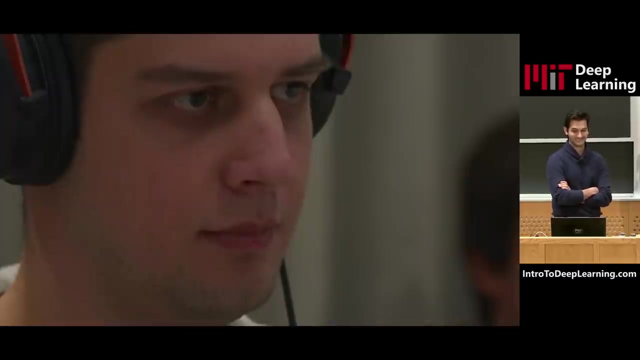 I wasn't expecting the AI to be that good. Everything that he did was proper, It was calculated and it was done well. I thought I'm learning something. Yes, Yes, It's much better than I expected it to be. I would consider myself a good player, right. 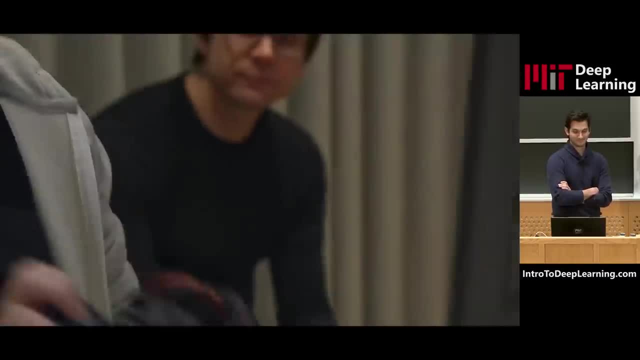 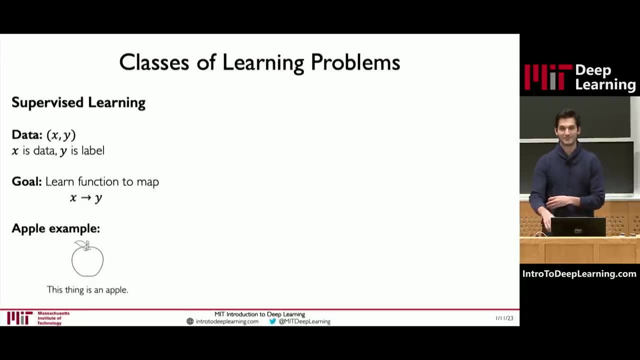 But I lost every single one of my games. We're way ahead of one, Right, so let's take maybe a start and take a step back, first of all, and think about how reinforcement learning fits into this whole paradigm of all of the different topics. 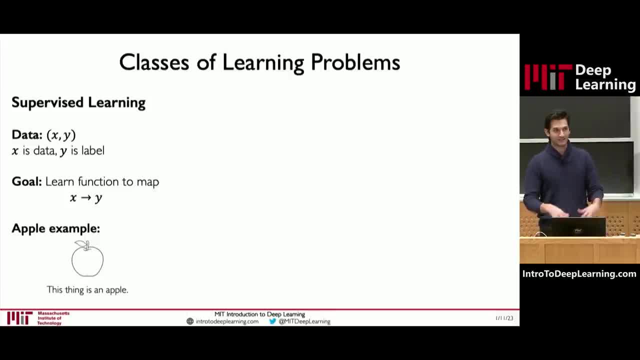 that you've been exposed to in this class so far. So as a whole, I think that we've really covered two different types of learning in this course to date. right Up until now, we've really started focusing in the beginning part of the lectures. 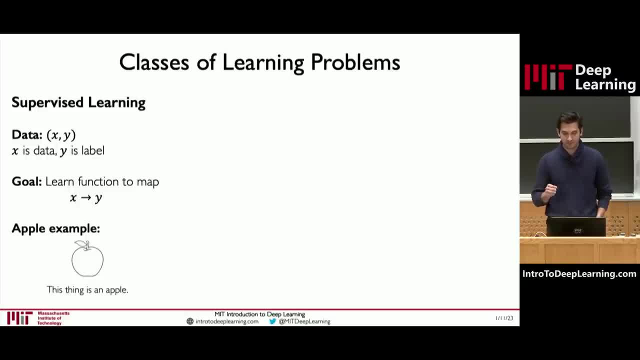 firstly, on what we called supervised learning right. Supervised learning is, in this domain where we're given data in the form of Xs, our inputs and our labels, Y right, And our goal here is to learn a function or a neural network that can learn to predict Y. 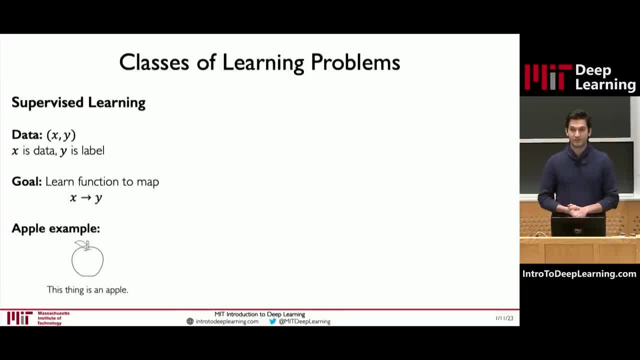 given our inputs X. So, for example, if you consider this example of an apple right, Observing a bunch of images of apples we want to detect in the future, if we see a new image of an apple, to detect that this is indeed an apple right. 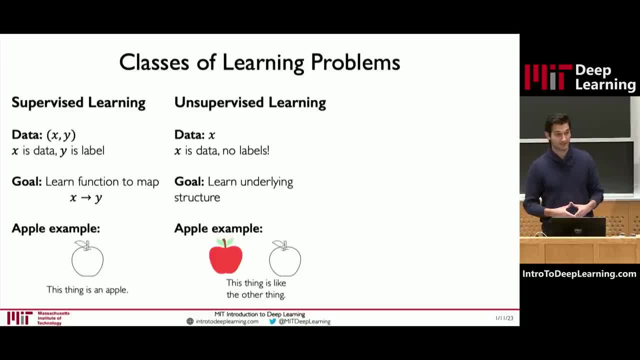 Now the second class of learning approaches that we've discovered yesterday, in yesterday's lecture, was that of unsupervised learning. In these algorithms, you have only access to the data. There's no notion of labels, right? This is what we learned about yesterday. 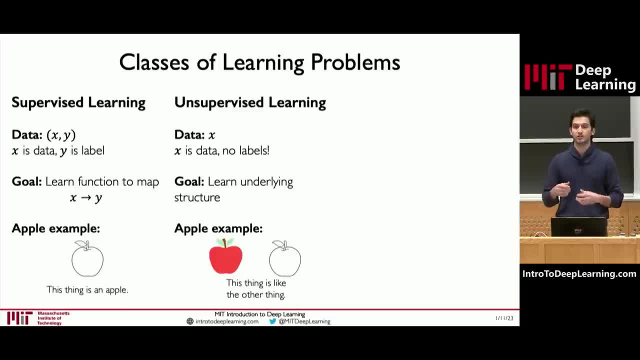 of algorithms. you're not trying to predict a label, but you're trying to uncover some of the underlying structure, what we were calling basically these latent variables, these hidden features in your data. so, for example, in this apple example, right using unsupervised learning, the analogous example would basically be to build a model that could understand and cluster certain certain parts. 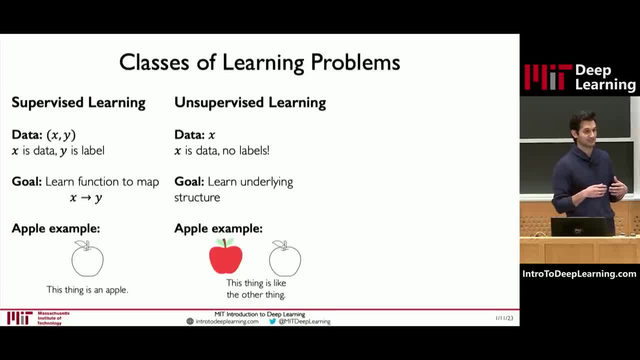 of these images together and maybe it doesn't have to understand that necessarily this is an image of an apple, but it needs to understand that you know this image of the red apple is similar. it has the same latent features and same semantic meaning as this black and white outline sketch of the apple. 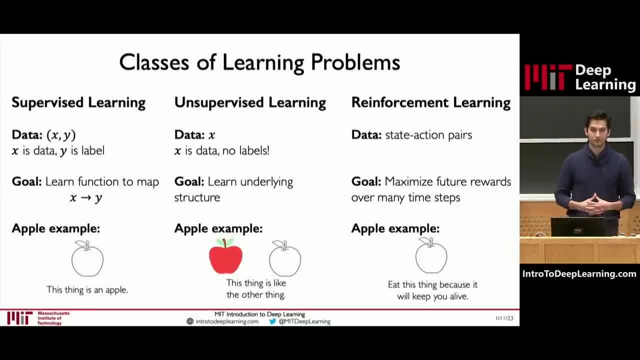 now, in today's lecture, we're going to talk about yet another type of learning algorithms. right, in reinforcement learning, we're going to be only given data in the form of what are called state action pairs. right now, states are observations. right, this is what the, the, the, 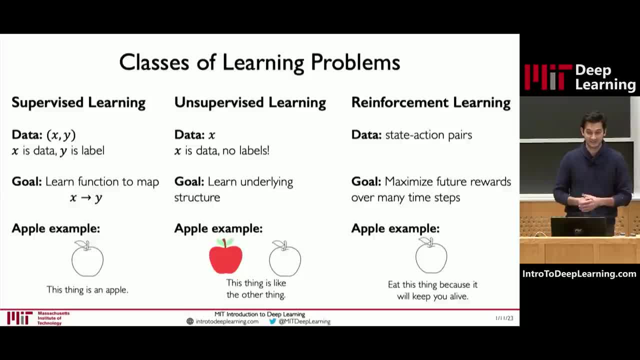 the- let's call it the neural network, is going to observe. it's what it sees. the actions are the behaviors that this agent takes in those particular states. so the goal of reinforcement learning is to build an agent that can learn how to maximize what are called rewards right. this is the third component. 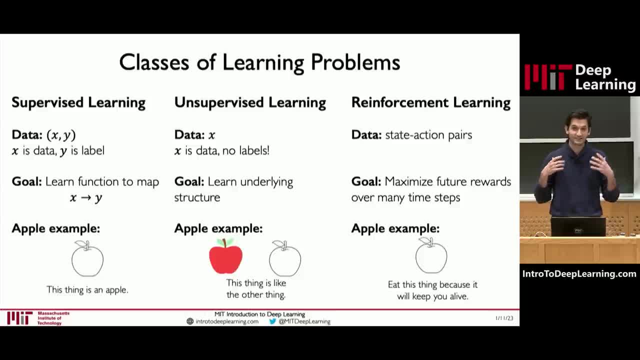 that is specific to reinforcement learning and you want to maximize all of those rewards over many, many time steps in the future. so again in this apple example, we might now see that the agent doesn't necessarily learn that okay, this is an apple or it looks like these other apples. now it has to learn to, let's say, eat the apple, take an action, eat that apple because it has learned that eating that apple makes it live longer or survive because it doesn't starve. 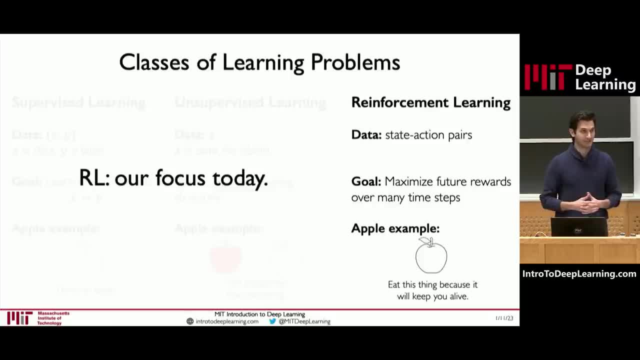 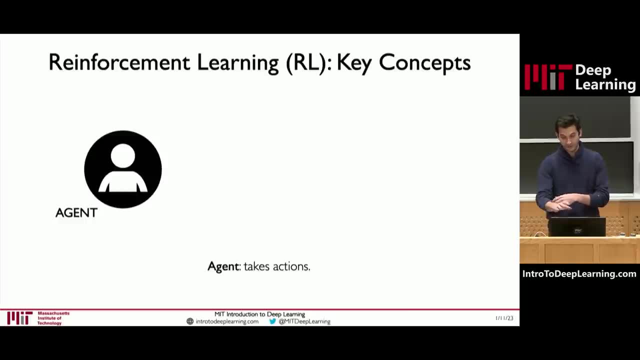 so in today, right like I said, we're going to be focusing exclusively on this third type of learning paradigm, which is reinforcement learning, and before we go any further, I just want to start by building up some very key terminology and like, basically, you know background for all of you, so that we're all on the same page when we start discussing some of the more complex components of today's lecture. so let's start by building up, you know, some of this terminology. the first main piece of terminology is that of an agent. right, an agent is a. 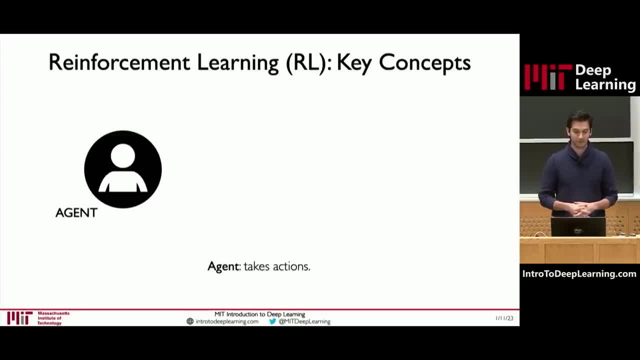 a being, basically, that can take actions. for example, you can think of an agent as as a machine, right, that is, let's say, an autonomous drone that is making a delivery of of, or, for example, in a game, it could be Super Mario that's navigating inside of. 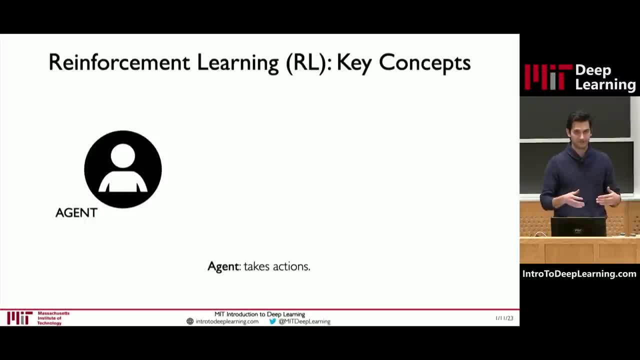 your video game, the algorithm itself. it's important to remember that the algorithm is the agent. right, we're trying to build an agent that can do these tasks and the algorithm is that agent. so in life, for example, all of you are agents. in life, the environment is the other kind of. 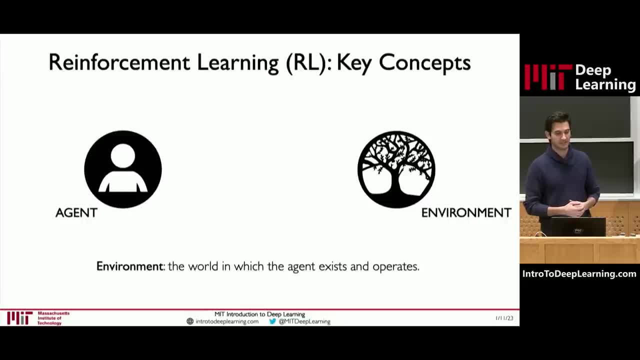 contrary approach or the contrary perspective to the agent. the environment is simply the world where that agent lives and where it operates right it, where it exists and it moves around in. the agent can send commands to that environment in the form of what are called actions, or it can take actions in. 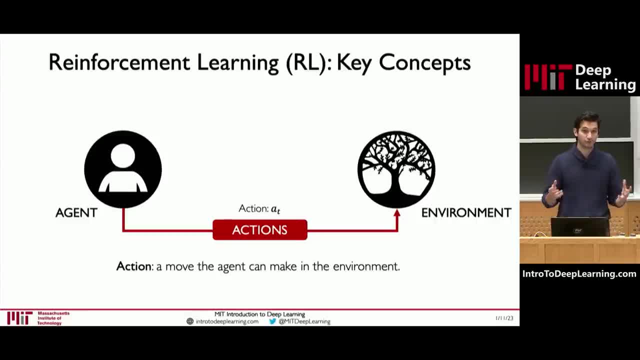 that environment and let's call for notation purposes. let's say, the possible set of all actions that it could take is, let's say, a set of capital, A right now. it should be noted that agents, at any point in time, could choose a ratio of absolutamente all the more dramatic or direct result versus the 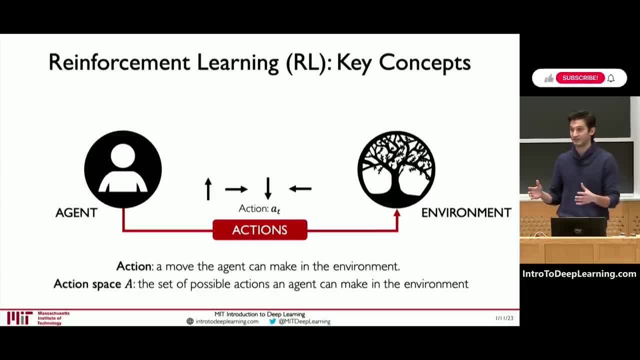 rate, you can have a green, ever brighter time of the human life and thus uh and able to to see generations on theто. that m is the way in which they can interpret them or make them all, the way Damen offend, or the way they can see their own. they can interpret their ownminuteshalido. agents S. therefore, it takes exactly that also. he canAA A to deal the story upside down. how you should move in all IP suffix and lets us the environment. You can see it now how the environment responds back to the agent, but the environment provides a 2030 long entityool variable and it's not that I don't know. 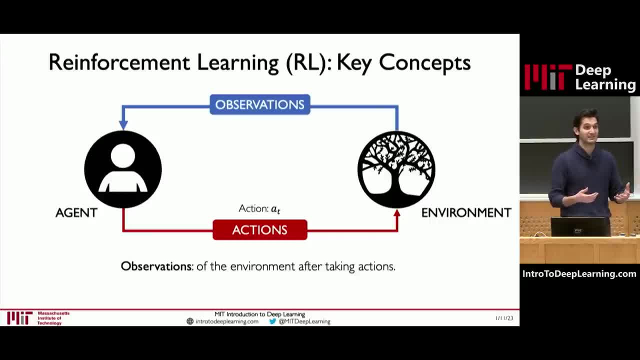 can tell the agent- you know what it should be seeing based on those actions that it just took- and it responds in the form of what is called a state. A state is simply a concrete and immediate situation that the agent finds itself in at that particular moment. Now it's important to remember. 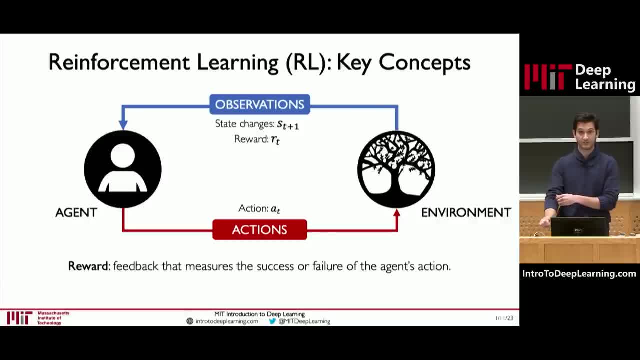 that, unlike other types of learning that we've covered in this course, reinforcement learning is a bit unique because it has one more component here, in addition to these other components, which is called the reward. Now, the reward is a feedback by which we measure, or we can try to. 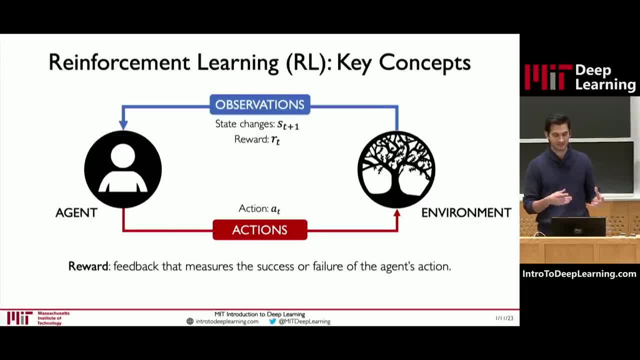 measure the success of a particular agent in its environment. So, for example, in a video game, when Mario grabs a coin, for example, he wins points right. So from a given state an agent can send out any form of actions to. you know, take some decisions and those 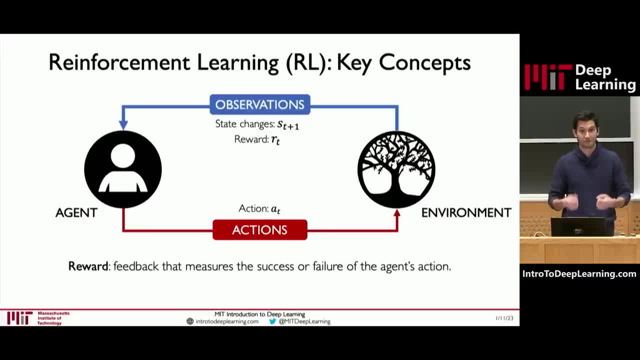 actions can be used to measure the success of a particular agent in its environment. Now it's also very important to remember that not all actions result in immediate rewards. You may take some actions that will result in a reward in a delayed fashion, maybe in a few time steps. 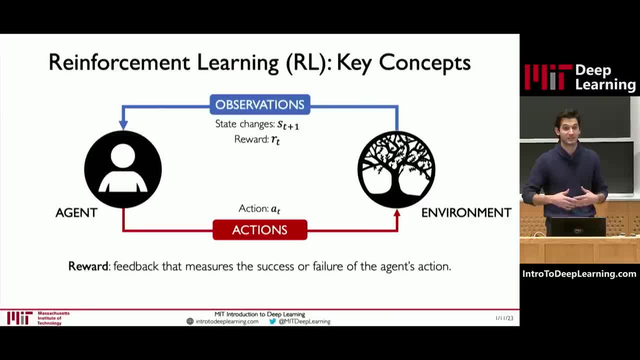 down the future, or maybe in life, maybe years, You may take an action today that results in a reward some time from now. right, But essentially all of these try to effectively evaluate some way of measuring the success of a particular action that an agent takes. So, for example, when we look 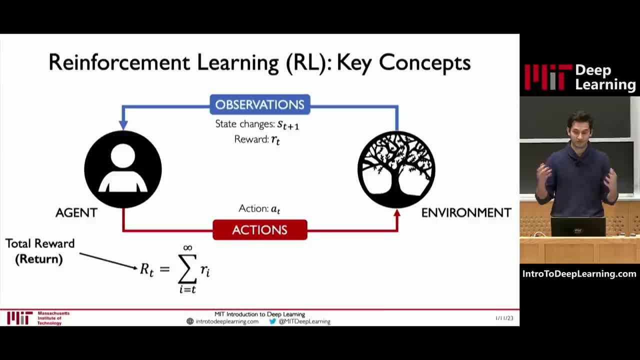 at the total reward that an agent accumulates over the course of its lifetime. we can simply sum up: all of the rewards that an agent gets after a certain time: t right. So this capital R of t is the sum of all rewards from that point on, into the future, into infinity. 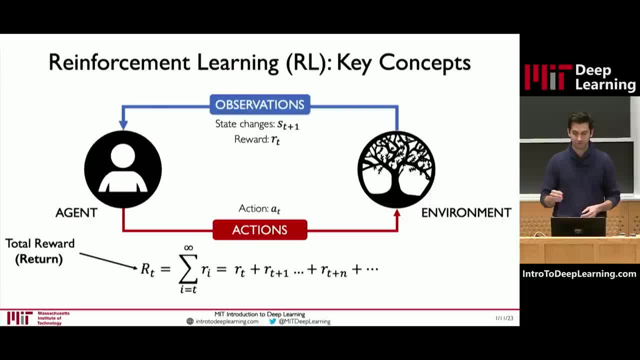 And that can be expanded to look exactly like this: Reward at time t plus the reward at time t plus 1 plus t plus 2, and so on and so forth. Often it's actually very useful for all of us to consider not only the sum of all of these. 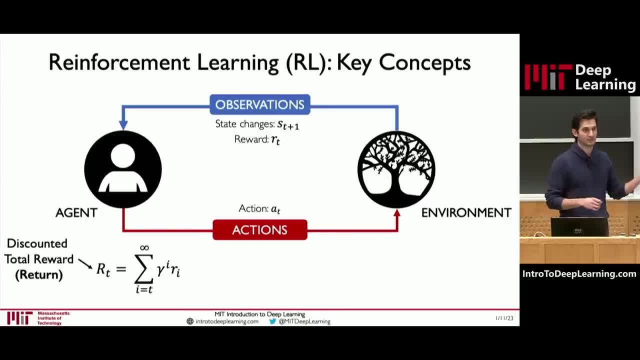 rewards, but instead what's called the discounted sum. So you can see, here I've added this gamma factor in front of all of the rewards and that discounting factor is essentially multiplied by every future reward that the agent sees, and it's discovered by the agent, And the reason that we 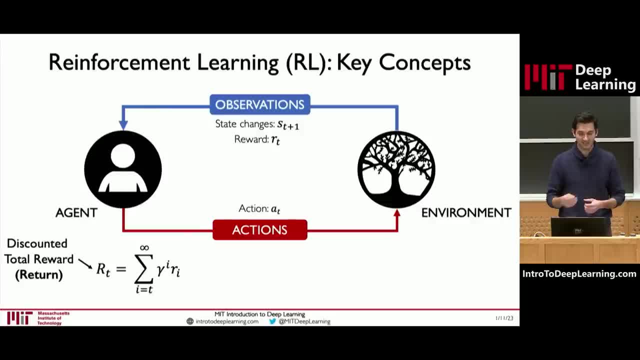 want to do this is actually to make sure that the reward that the agent sees is actually multiplied by the reward that the agent sees. So this dampening factor is designed to make future rewards essentially worth less than rewards that we might see at this instant, at this moment, right. 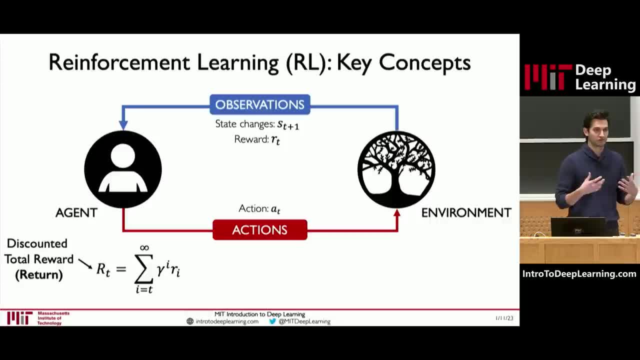 now. Now you can think of this as basically enforcing some kind of short-term greediness in the algorithm, right? So, for example, if I offered you a reward of $5 today or a reward of $5 in 10 years from now, I think all of you would prefer that $5 today, simply because you know. 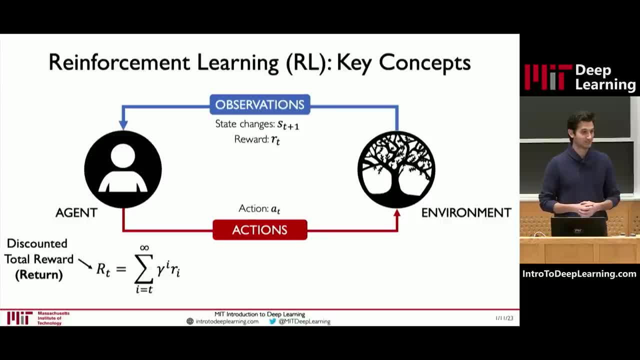 we have that same discounting factor applied to this processing right. We have that factor that that $5 is not worth as much to us if it's given to us 10 years in the future, and that's exactly how this is captured here as well. mathematically, This discounting factor is like, like I said, 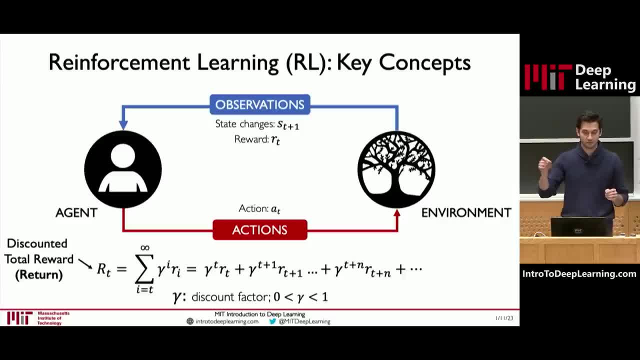 multiplied at every single future reward exponentially, and it's important to understand that also. typically this discounting factor is, you know, between zero and one. There are some exceptional cases where maybe you want some discounting factor and you want some discounting factor. 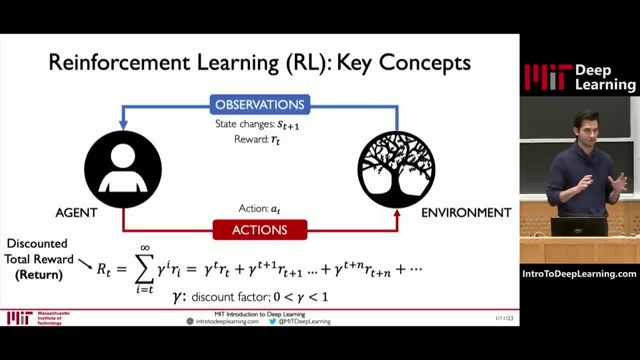 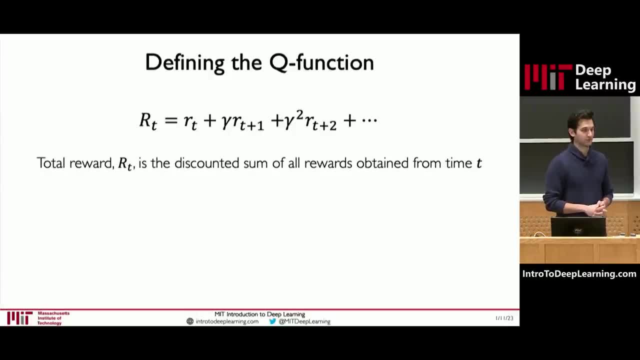 greater than one, but in general, that's not something we're going to be talking about today. Now, finally, it's very important in reinforcement learning this special function called the Q function, which ties in a lot of these different components that I've just shared with you. 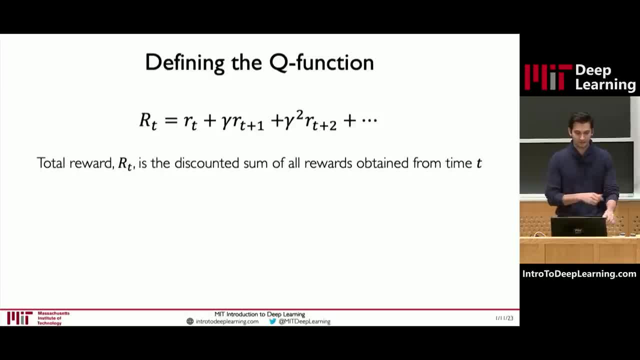 all together. Now let's look at what this Q function is right. So we already covered this R of T function right. R of T is the discounted sum of rewards from time t all the way into the future, into time infinity. But remember that this R of T right it's. 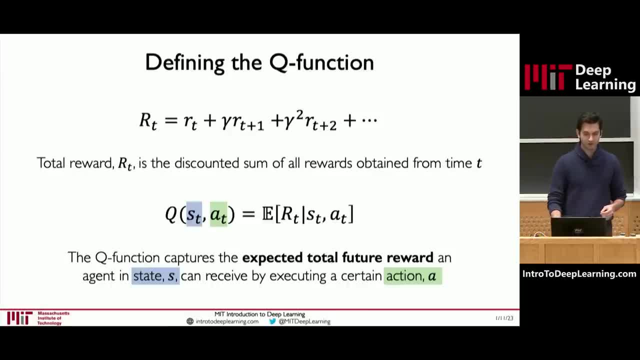 discounted number one and number two. we're going to try and build a Q function that captures the maximum or the best action that we could take that will maximize this reward. So let me say that one more time, in a different way. The Q function takes as input two different things. 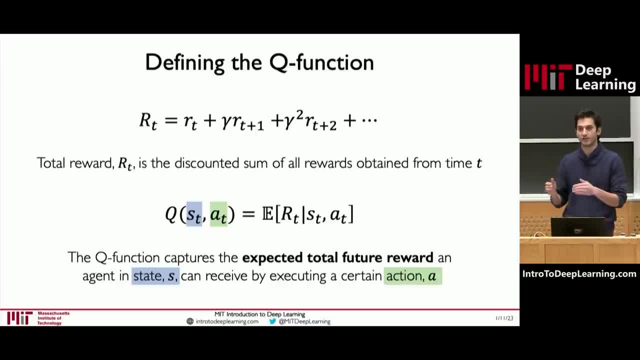 The first is the state that you're currently in and the second is a possible action that you could execute in this particular state. So here S of T is that state at time t. A of T is that action that you may want to take at time t. 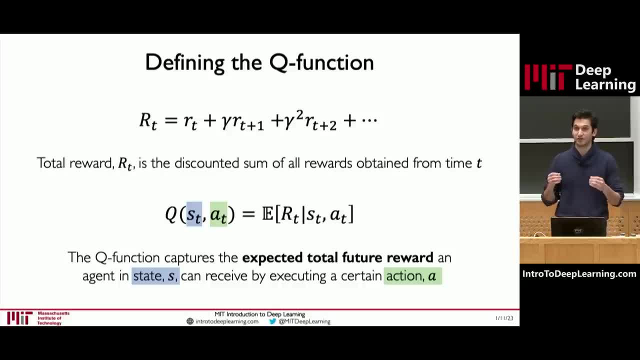 and the Q function of these two pieces is going to denote or capture what the expected total return would be of that agent if it took that action in that particular state. Now, one thing that I think maybe we should all be asking is how do we know that the Q function is going to capture the 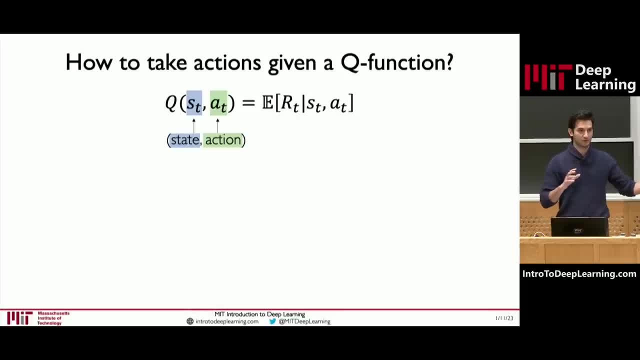 maximum or the best action that we could take in this particular state. So what we're asking ourselves now is: this seems like a really powerful function, right? If you had access to this type of a function, this Q function, I think you could actually perform a lot of tasks right off the bat. 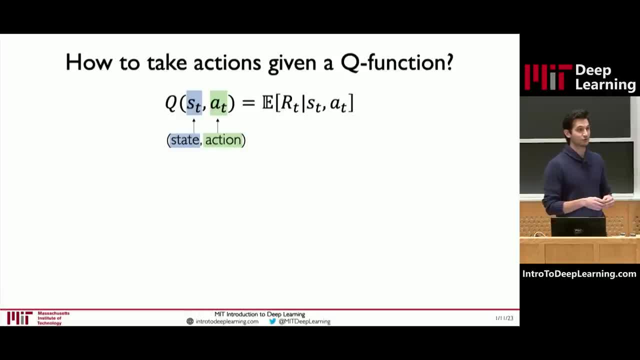 right. So if you wanted to, for example, understand how to what actions to take in a particular state, and let's suppose I gave you this magical Q function, does anyone have any ideas of how you could transform that Q function to directly infer what action should be taken? 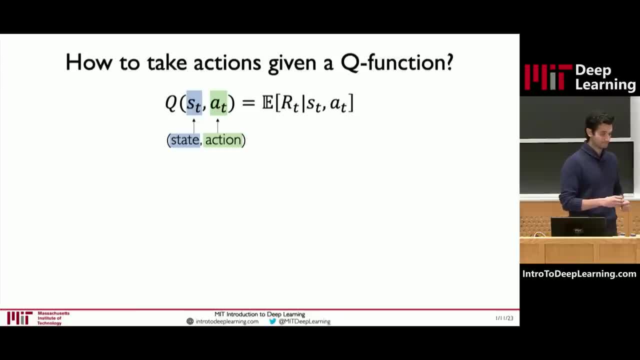 Given a state, you can look at your possible action space and pick the one that gives you the highest Q value. Exactly So, that's exactly right. So just to repeat that one more time: the Q function tells us for any possible action, right? what is the expected reward for that action? 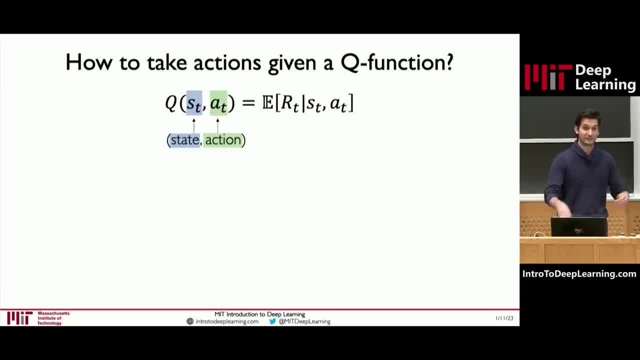 to be taken. So if we wanted to take a specific action given a specific state, ultimately we need to, you know, figure out which action is the best action. The way we do that from a Q function is simply to pick the action that will maximize our future reward, and we can simply try out: number. 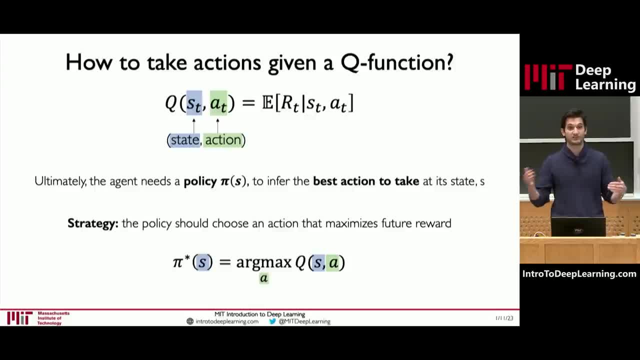 one. if we have a discrete action space, we can simply try out all possible actions, compute their Q value for every single possible action, based on the state that we currently find ourselves in, and then we pick the action that is going to result in the highest Q value. If we have a 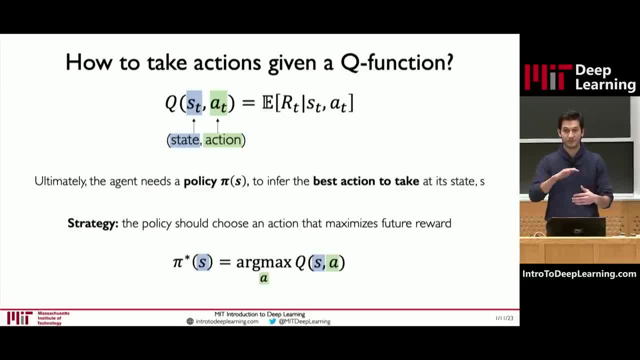 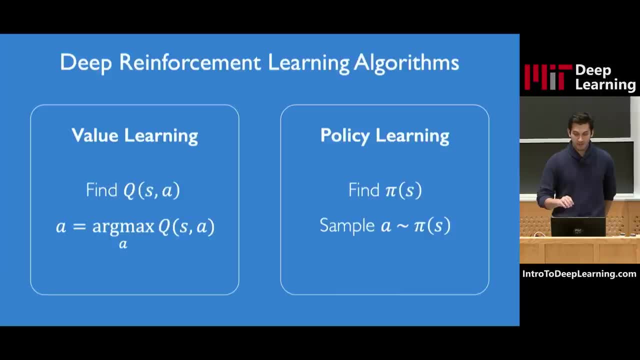 continuous action space. maybe we do something a bit more intelligent, maybe following the gradients along this Q value curve And maximizing it as part of an optimization procedure. But generally in this lecture, what I want to focus on is actually how we can obtain this Q. 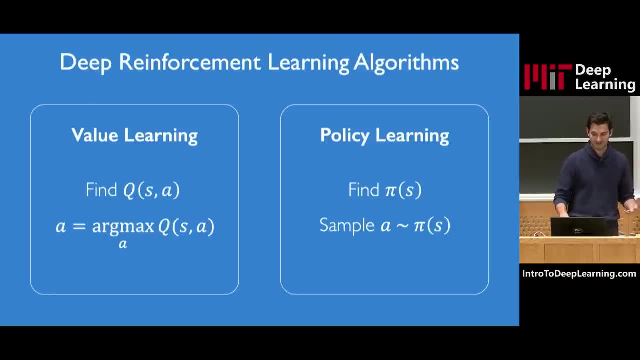 function to start with right. I kind of skipped a lot of steps in that last slide where I just said: let's suppose I give you this magical Q function. how can you determine what action to take? But in reality we're not given that Q function. We have to learn that Q function using deep. 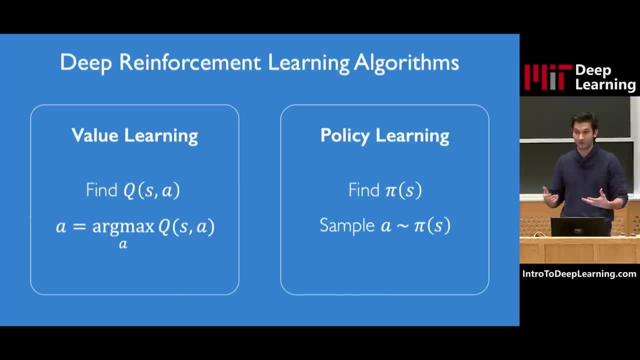 learning, And that's what today's lecture is going to be talking about primarily- is, first of all, how can we construct and learn that Q function? How can we construct and learn that Q function? How can we construct and learn that Q function from data? And then, of course, the final step is use that Q function to you know. 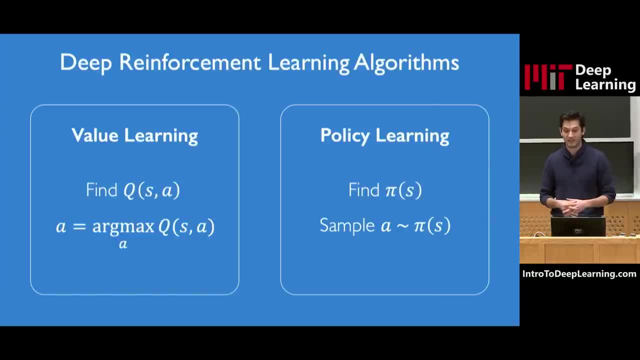 take some actions in the real world And, broadly speaking, there are two classes of reinforcement learning algorithms that we're going to briefly touch on as part of today's lecture. The first class is what's going to be called value learning, And that's exactly this process that we've just talked about. Value learning tries to estimate our Q function right. 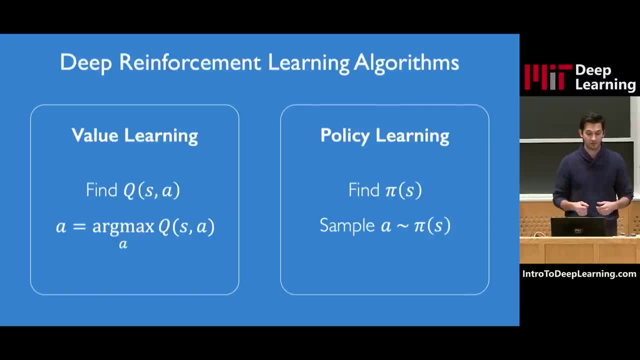 So to find that Q function, Q, given our state and our action, and then use that Q function to you know, optimize for the best action to take given a particular state, that we find ourselves in The second class of algorithms, which we'll touch on right at the end of today's lecture, is kind of a different framing of the 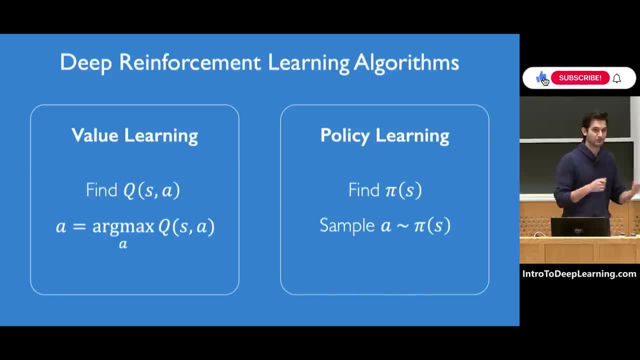 same approach, But instead of first optimizing the Q function and finding the Q value, and then using that Q function to optimize our actions, what if we just tried to directly optimize our policy, which is what action to take based on a particular state that we find ourselves in? 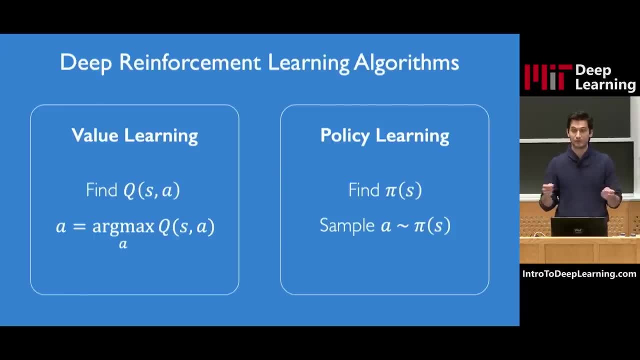 If we do that, if we can obtain this function right, Then we can directly sample from that policy distribution to obtain the optimal action. We'll talk more details about that later in the lecture. But first let's cover this first class of approaches, which is Q learning approaches. 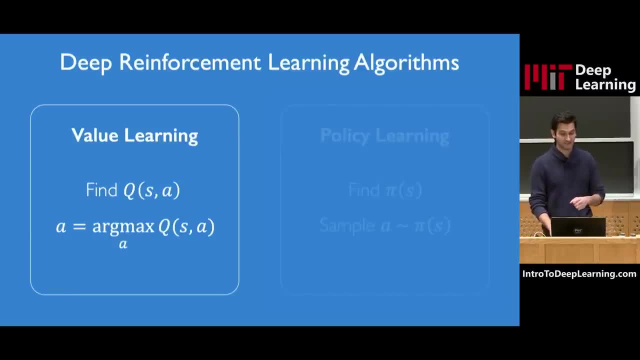 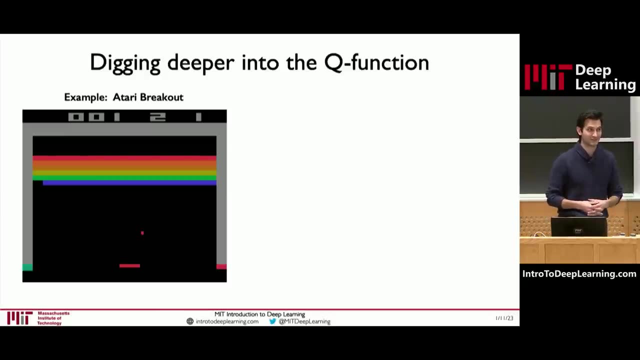 And we'll build up that intuition and that knowledge onto the second part of policy learning. So maybe let's start by just digging a bit deeper into the Q function specifically, just to start to understand. you know how we could estimate this in the beginning. 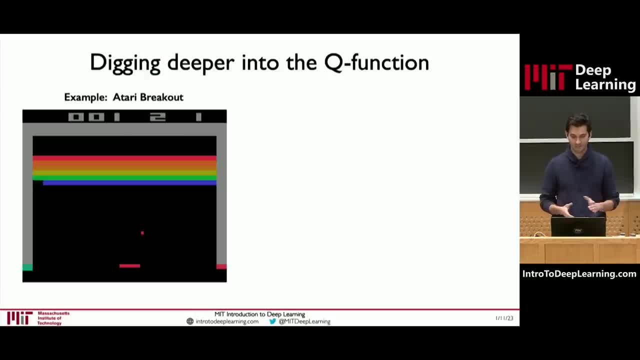 The first, let me introduce this game. Maybe some of you recognize it. This is the game called Atari Breakout. The game here is essentially one where the agent is able to move left or right this paddle on the bottom, left or right, And the objective is to move it in a way that this ball that's coming down towards the bottom of the screen can be, you know, bounced off of your paddle, reflected back up, And essentially you want to break out right, reflect that ball back up to the top of the screen, towards the rainbow portion, and keep it moving. 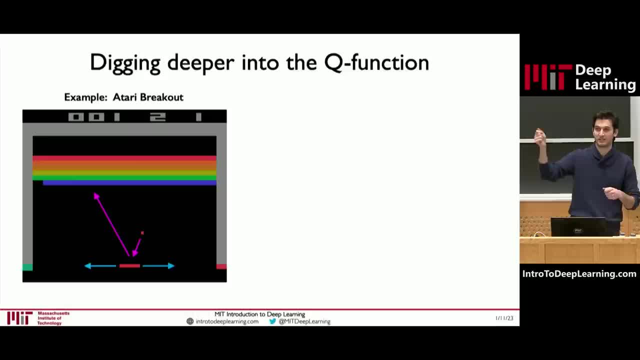 And then keep breaking off. Every time you hit a pixel on the top of the screen, you break off that pixel. The objective of the game is to basically eliminate all of those rainbow pixels, right? So you want to keep hitting that ball against the top of the screen until you remove all the pixels. 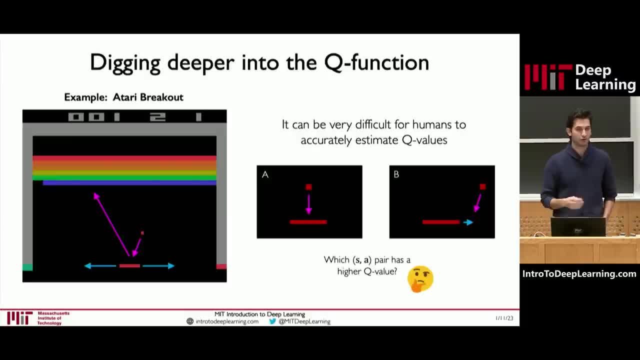 Now the Q function tells us, you know, the expected total return, or the total reward that we can expect, based on a given state and action pair that we may find ourselves in this game. Now the first point I want to make here. 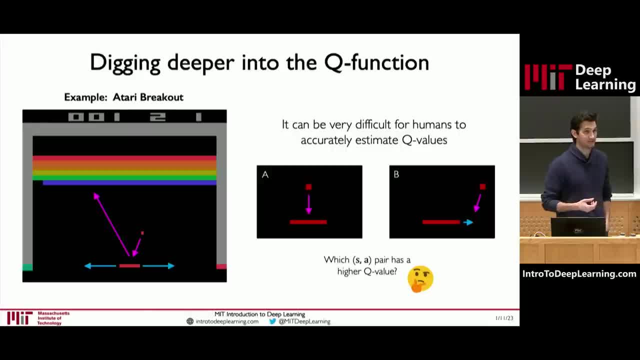 is that sometimes, even for us as humans, to understand what the Q value should be is sometimes quite unintuitive, right? So here's one example. Let's say we find these two state action pairs right. Here is A and B, two different options that we can be presented with in this. 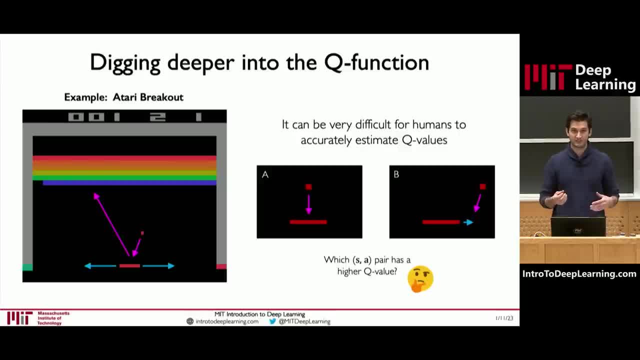 game A. the ball is coming straight down towards us. That's our state. Our action is to do nothing and simply reflect that ball back up, vertically up. The second situation. the state is basically that the ball is coming slightly at an angle. We're not quite underneath it yet and we need 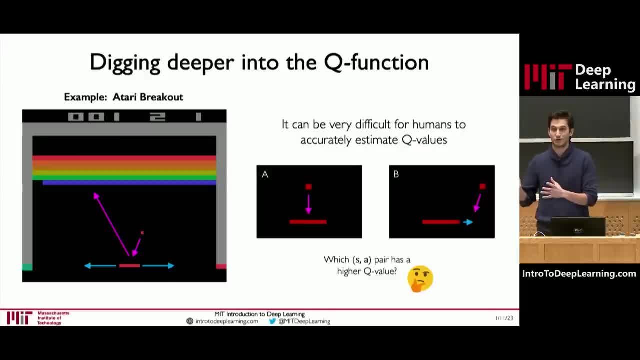 to move towards it and actually hit that ball in a way that you know we'll make it and not miss it. hopefully, right, So hopefully that ball doesn't pass below us. then the game would be over. Can you imagine, you know, which of these two options might have a higher Q value? 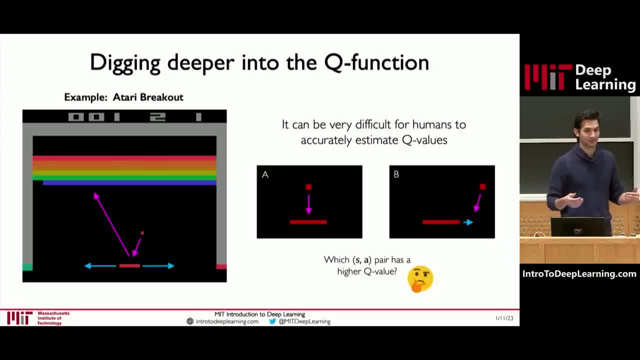 For the network? which one would result in a rate of reward for the neural network or for the agent? So how many people believe A would result in a higher return? Okay, How about B? Okay, How about someone who picked B? Can you tell me why B? 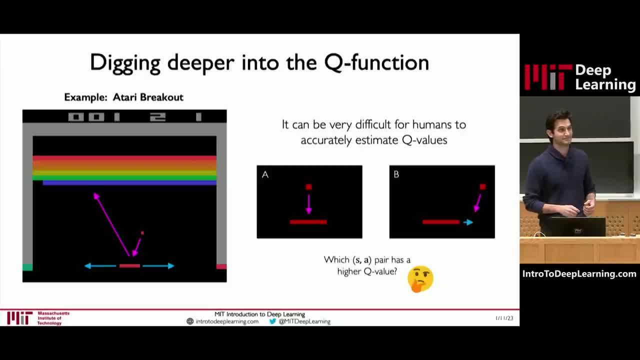 Why is agency? You're actually doing something, Okay, Yeah, How about more For the first one? For A you only have like the maximum you can take off is like one, because after you reflect, your automatic comes back down. but then B you can bounce around and there's more than one at. 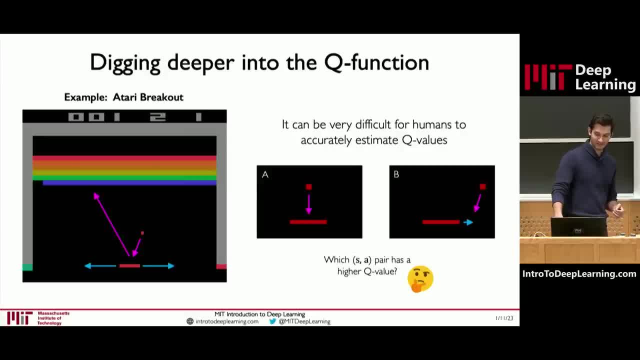 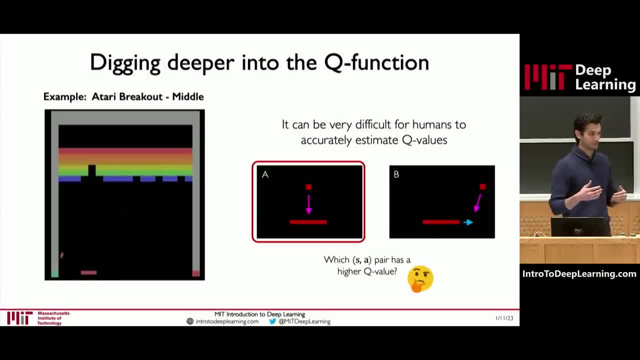 least Exactly, And actually there's a very interesting thing. So when I first saw this, actually it was very unintuitive for me why A is actually working much worse than B, But in general this very conservative action of B, you're kind of exactly like you said. The two answers were: 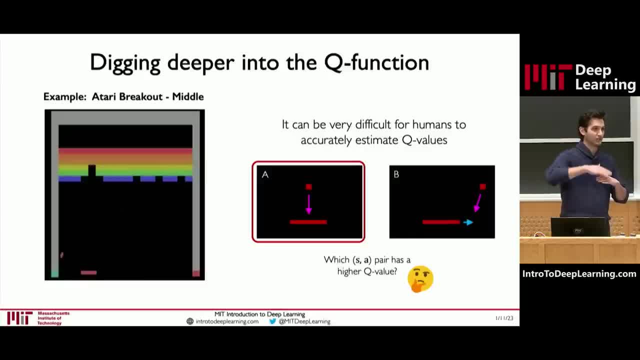 implying is that A is a very conservative action. You're kind of only going up and down. It will achieve a good reward. It will solve the game right. In fact it solves the game exactly like this right here. You can see, in general, this action is going to be quite conservative, It's. 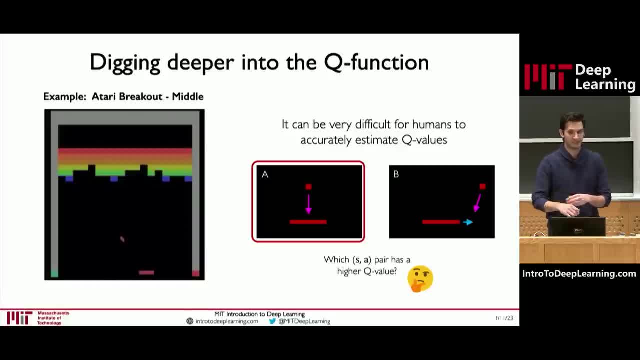 just bouncing up, hitting one point at a time from the top and breaking off very slowly the board that you can see here. But in general you see, the part of the board that's being broken off is towards the center of the board, right, Not much on the edges of the board. If you look at B, 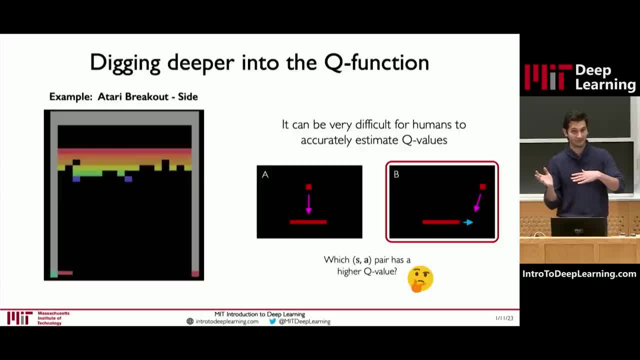 now with B, you're kind of having agency, like one of the answers said. You're coming towards the ball And what that implies is that you're sometimes going to actually hit the corner of your paddle and have a very extreme angle on your paddle and hit the sides of the board as well. 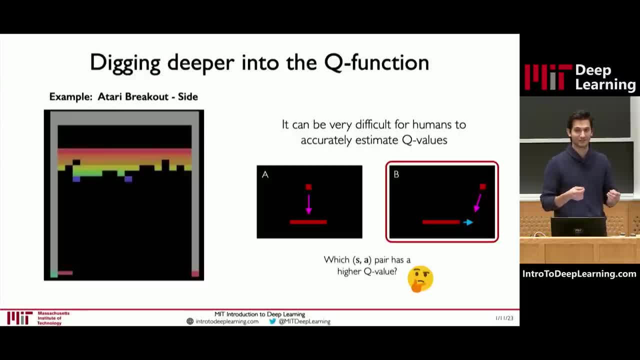 And it turns out that the algorithm, the agent, can actually learn that hitting the side of the board can have some kind of unexpected consequences that look like this. So here you see it trying to enact that policy. It's targeting the sides of the board, But once you get to the bottom of the board, 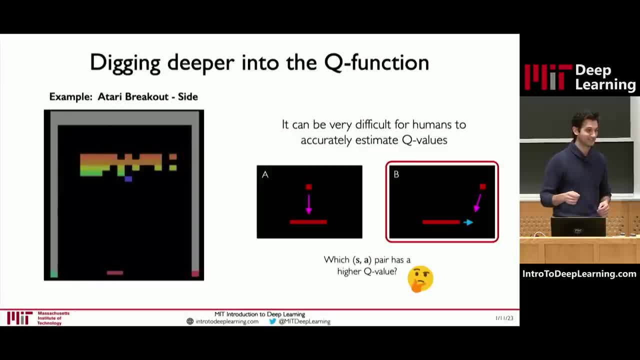 once it reaches a breakout on the side of the board. it found this hack in the solution where now it's breaking off a ton of points. So that was a kind of a trick that this neural network learned, which was a way that it even moves away from the ball as it's coming down, just so it could move. 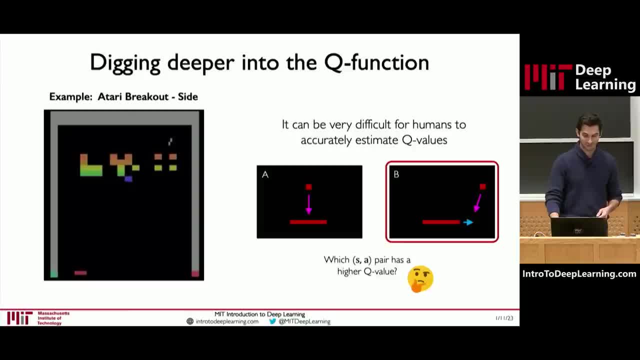 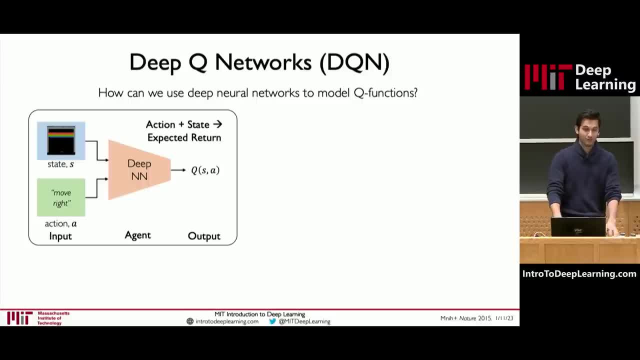 back towards it, just to hit it on the corner and execute on those corner parts of the board and break out a lot of pieces for free, almost. So now that we can see that sometimes obtaining the Q function can be a little bit uninteresting, it can be a little bit difficult, but it can also be. 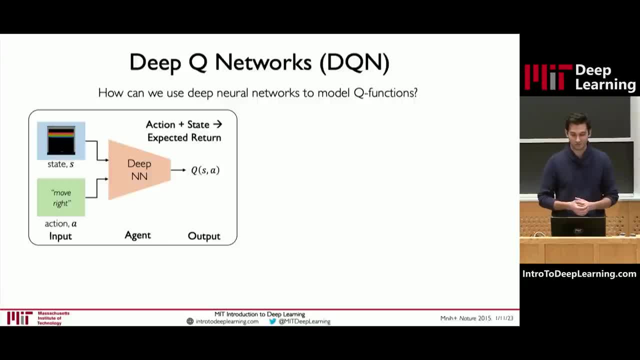 a little bit unintuitive, But the key point here is that if we have the Q function, we can directly use it to determine, you know, what is the best action that we can take in any given state that we find ourselves in. So now the question naturally is: how can we train a neural network that can 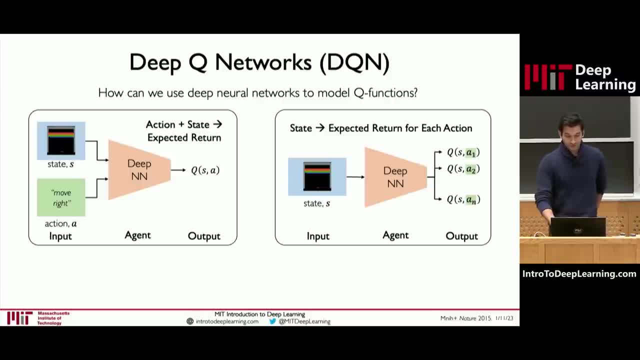 indeed learn this Q function. So the type of the neural network here. naturally, because we have a function that takes as input two things. let's imagine our neural network will also take as input two things, right? So it's going to be the state of the board. You can think of this as simply the 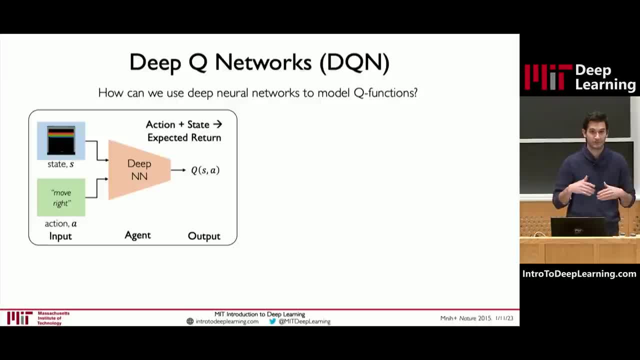 pixels that are on the screen describing that board. So it's an image of the board at a particular time. Maybe you want to even provide two or three images to give it some sense of temporal information and some past history as well. But all of that information can be combined together and provided. 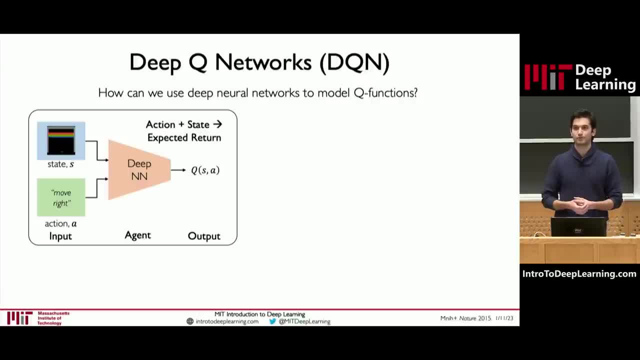 to the network in the form of a state, And in addition to that, you may also want to provide it some actions as well, right? So in this case, the actions that a neural network or an agent could take in this game is to move to the right, to the left, to stay still right, And those could be three different. 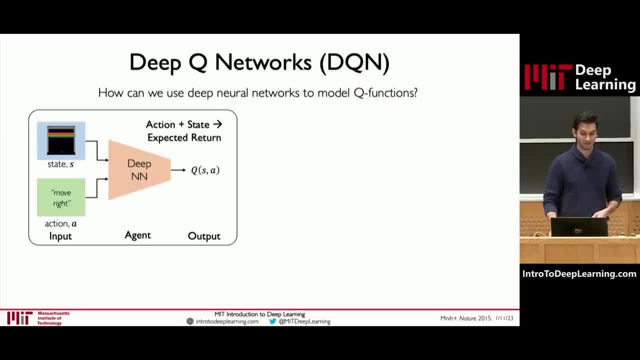 actions that could be provided and parameterized to the input of a neural network. The goal here is to, you know, estimate the single number output that measures what is the expected value, or the expected Q value of this neural network at this particular state action pair. Now, oftentimes, 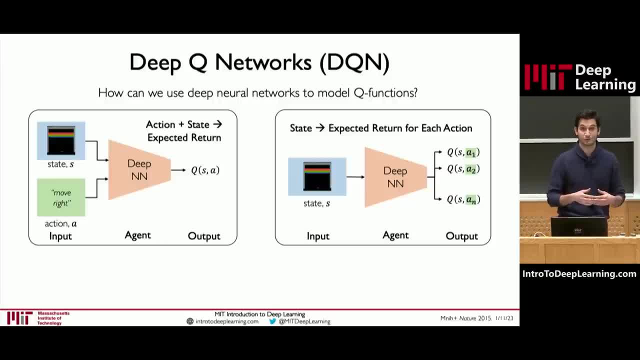 what you'll see is that if you wanted to evaluate- let's suppose- a very large action space, it's going to be very inefficient to try the appropriate approach on the left with a very large action space, because what it would mean is that you'd 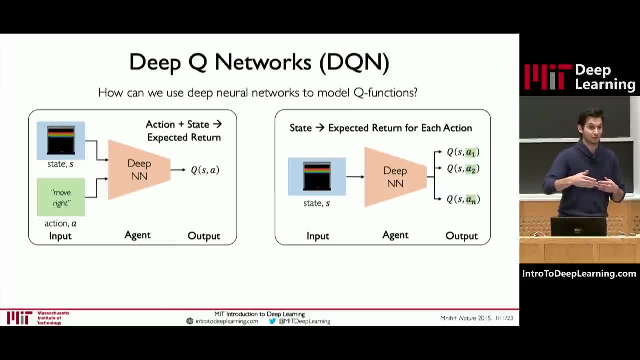 have to run your neural network forward many different times, one time for every single element of your action space. So what if, instead, you only provided it an input of your state and as output you gave it, let's say, all n different Q values. one Q value for every. 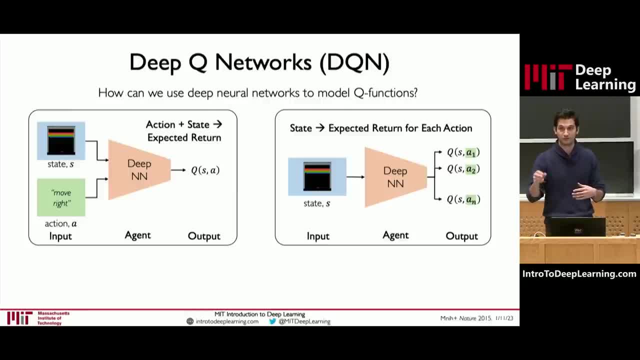 single possible action. That way you only need to run your neural network once for the given state that you're in, and then that neural network will tell you, for all possible actions, what's the maximum. You could simply then look at that output and pick the action that has the chi. 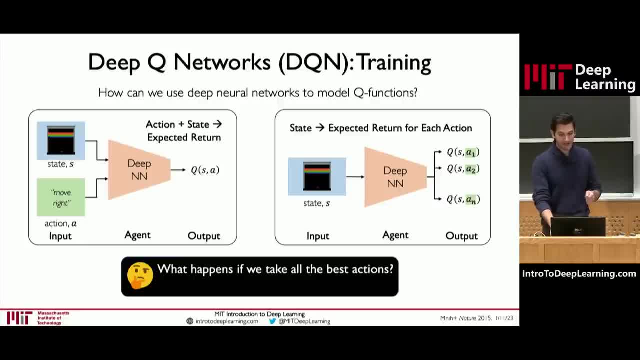 as Q value. Now what would happen, right? so actually, the question I want to pose here is really: you know, we want to train one of these two networks. Let's stick with the network on the right for simplicity, just since it's a much more efficient version of the network on the left. 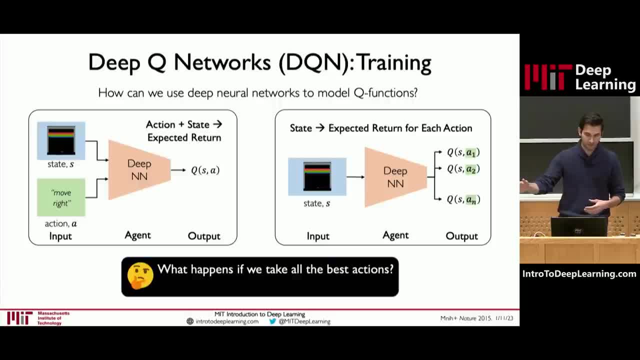 And the question is: you know how do we actually train that network on the right? And specifically, I want all of you to think about really the best case scenario just to start with, how an agent would perform ideally in a particular 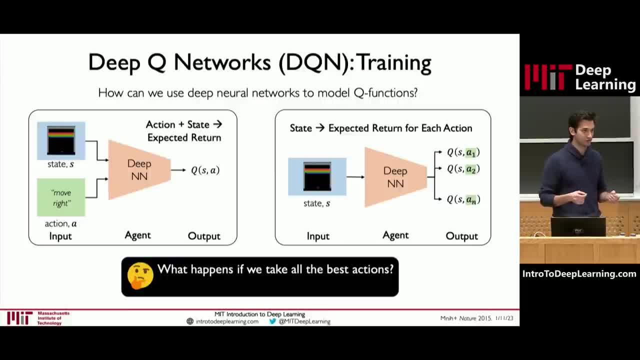 situation or what would happen right if an agent took all of the ideal actions at any given state. This would mean that, essentially, the target return right, the predicted or the value that we're trying to predict- the target is going to always be maximized right And this can serve. 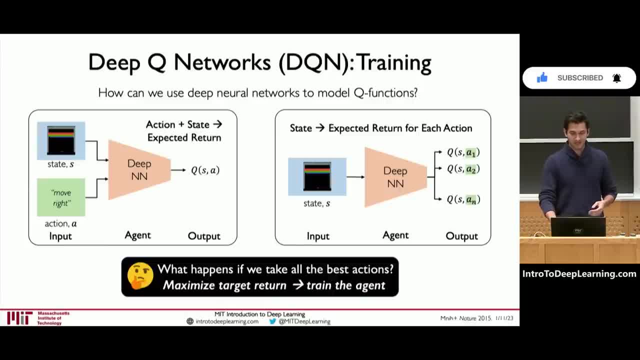 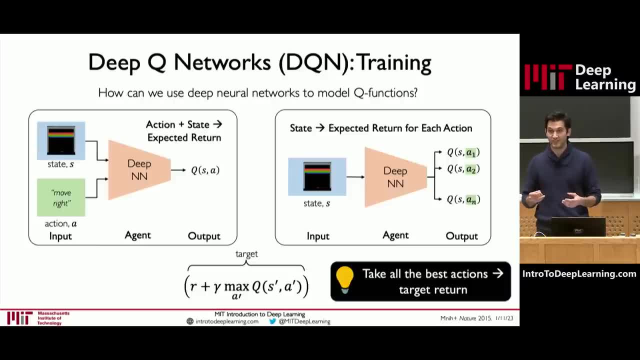 as essentially the ground truth to the agent. Now, for example, to do this, we want to formulate a loss function that's going to essentially represent our expected return if we're able to take all of the best actions right. So, for example, if we select an initial reward, 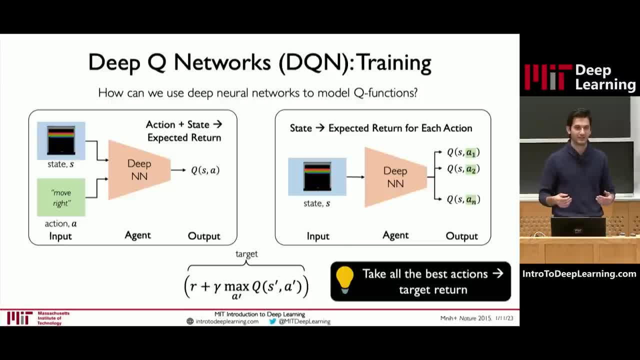 plus selecting some action in our action space that maximizes our expected return. then for the next future state we need to apply that discounting factor and recursively apply the same equation And that simply turns into our target right Now we can ask basically: 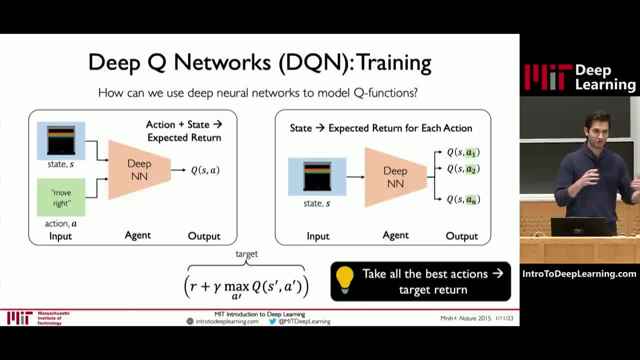 what does our neural network predict right? So that's our target and we recall from previous lectures. if we have a target value- in this case our Q value- is a continuous variable. we have also a predicted variable that is going to come as part of the output of every single one. 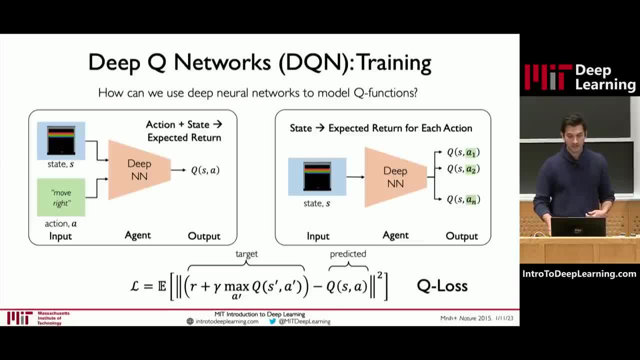 of these potential actions that could be taken, we can define what's called a Q loss, which is essentially just a very simple mean squared error loss between these two continuous variables. We minimize their distance. So what we're going to do is we're going to look at this model over two, over many, many different. 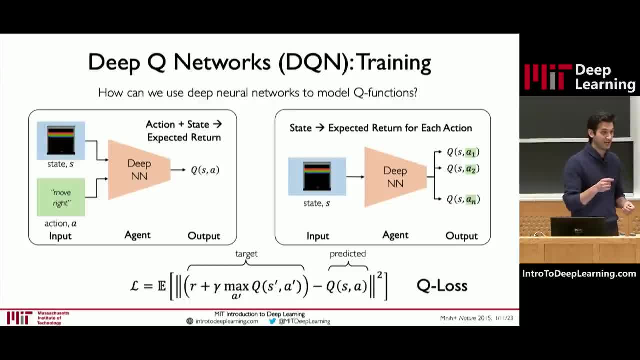 iterations of applying our neural network in this environment, observing actions. and observing not only the actions but, most importantly, after the action is committed or executed we can see exactly the ground truth expected return right. So we have the ground truth labels to train and 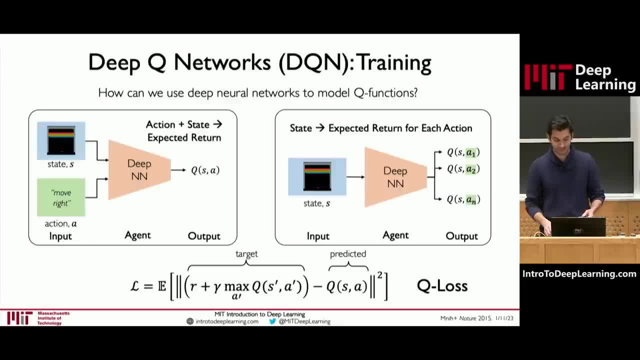 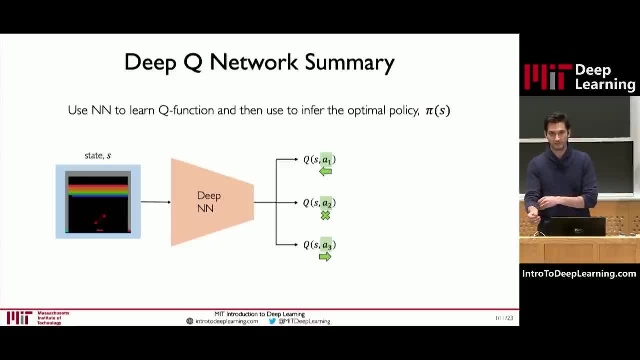 supervise this model directly from the actions that were executed as part of random selection, for example. Now let me just stop right there and maybe summarize the whole process one more time in maybe a bit different terminology, just to give everyone kind of a different perspective. 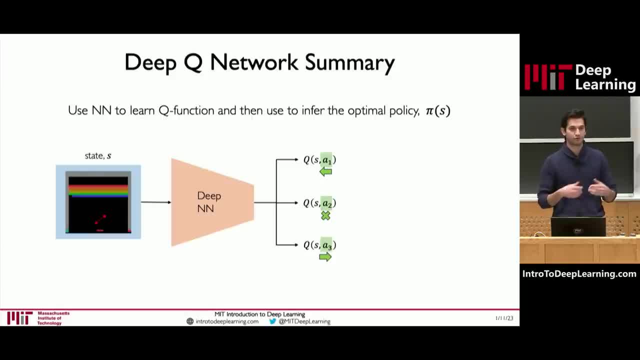 on this same problem. So our deep neural network that we're trying to train looks like this right: It takes as input a state, it's trying to output n different numbers. those n different numbers correspond to the Q value associated to n different actions. one Q value per action. Here the actions in Atari are represented by the student network and the Q value is represented in the actions that are in the system. Here the actions in Atari are represented by the Q value associated to the N different actions. one Q value per action. 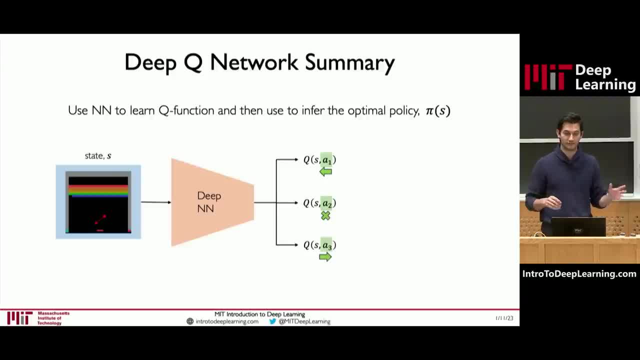 breakout, for example, should be three actions. we can either go left, we can go right or we can do nothing. we can stay where we are right. so the next step from this we saw, if we have this Q value output, what we can do with it is we can make an action or we can even. let me be more. 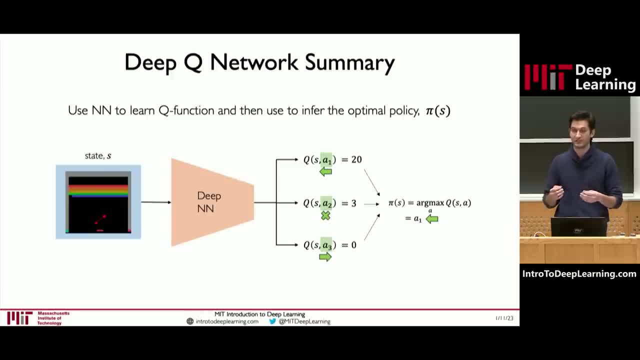 formal about it. we can develop what's called a policy function. a policy function is a function that, given a state, it determines what is the best action. so that's different than the Q function, right, the Q function tells us, given a state, what is the best, or what is the value, the return of 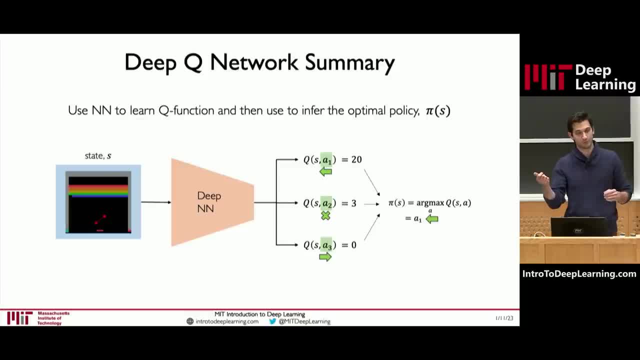 every action that we could take. the policy function tells us one step more than that: given an, given a state, what is the best action? right? so it's a very end-to-end way of thinking about, you know, the agent's decision-making process. based on what I see right now, what is the action? 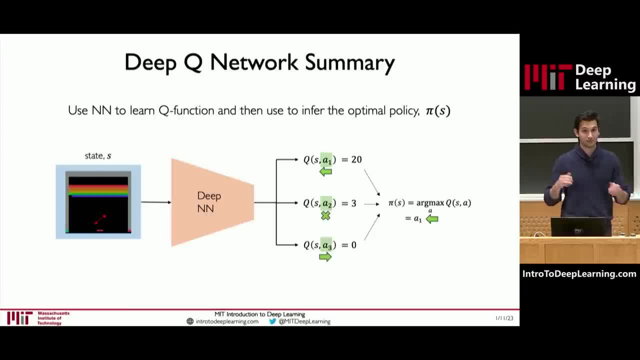 that I should take and we can determine that policy function is a policy function that we can develop. and we can determine what is the best action if we can take the policy function directly from the Q function itself, simply by maximizing and optimizing all of the different Q values for all of the different actions that we see here. 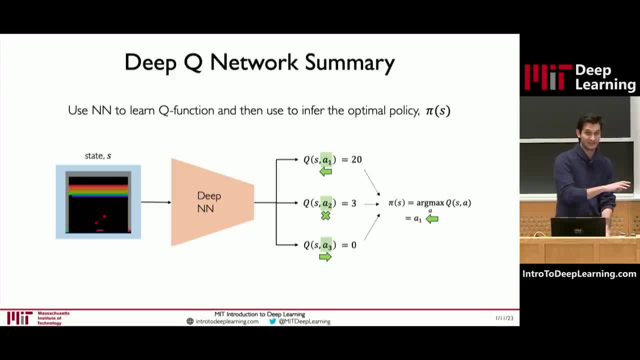 so, for example, here we can see that, given this state, the Q function has the result of these three different values, has a Q value of 20 if it goes to the left, has a Q value of 3, it stays in the same place and it has a Q value of zero. it's going to basically die after this iteration. 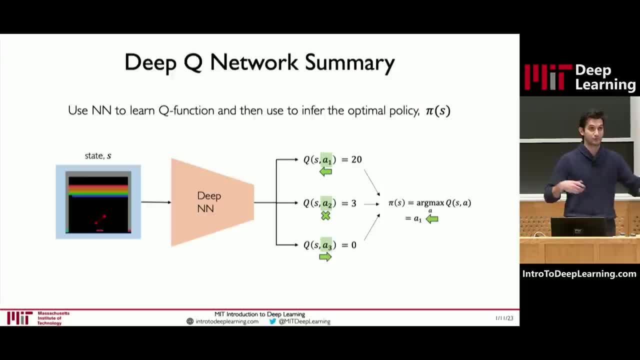 if it moves to the right, because you can see that the ball is coming to the left, left of it. if it moves to the right, the game is over, right. So it needs to move to the left in order to do that, in order to continue the game, and the Q value reflects that. 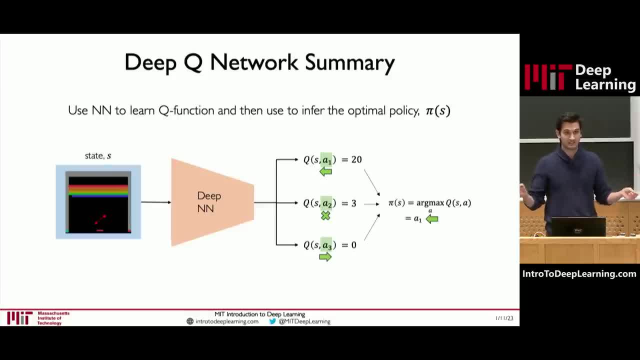 The optimal action here is simply going to be the maximum of these three Q values- In this case it's going to be 20, and then the action is going to be the corresponding action that comes from that 20, which is moving left. Now we can send this action back to the environment. 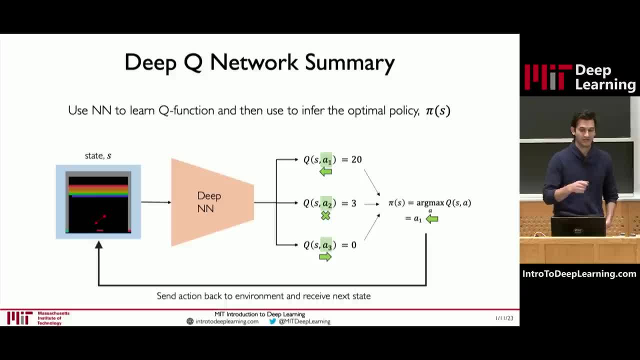 in the form of the game to execute the next step right. And as the agent moves through this environment, it's going to be responded with not only by new pixels that come from the game but, more importantly, some reward signal. Now it's very important to remember that the reward 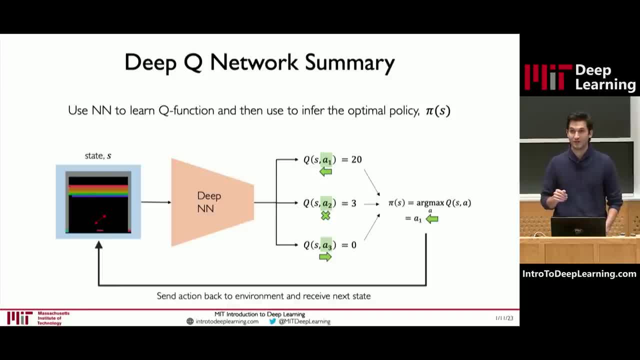 signals in Atari Breakout are very sparse. right, You get a reward not necessarily based on the action that you take at this exact moment. It usually takes a few time steps for that ball to travel back up to the target top of the screen, so usually your rewards will be quite delayed, maybe at least by several time. 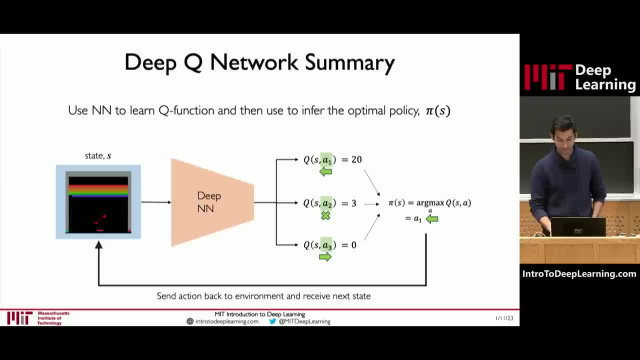 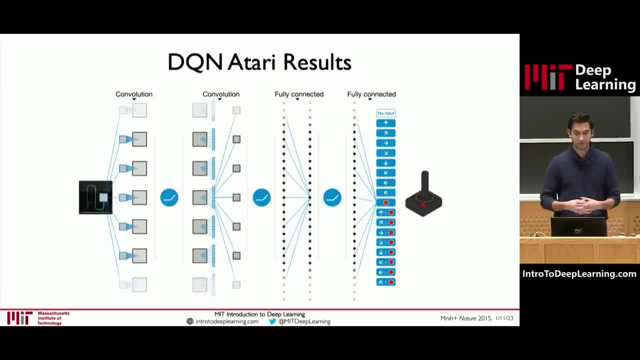 steps, sometimes even more if you're bouncing off of the corners of the screen. Now, one very popular or very famous approach that showed this was presented by DeepMind- Google DeepMind- several years ago, where they showed that you could train a Q value network and you can see. 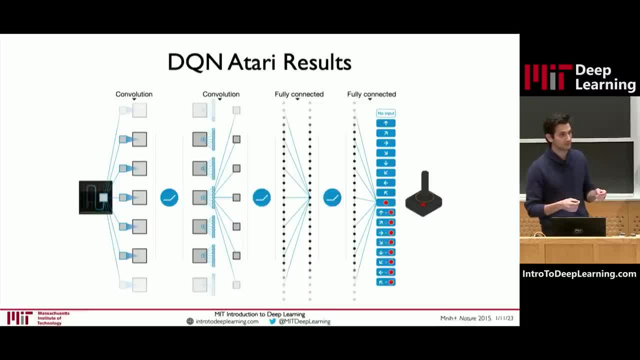 the input on the left-hand side is simply the raw pixels coming from the screen all the way to the action that you take at the top of the screen. So if you're bouncing off of the screen, you could train the actions of a controller on the right-hand side and you could train this one. 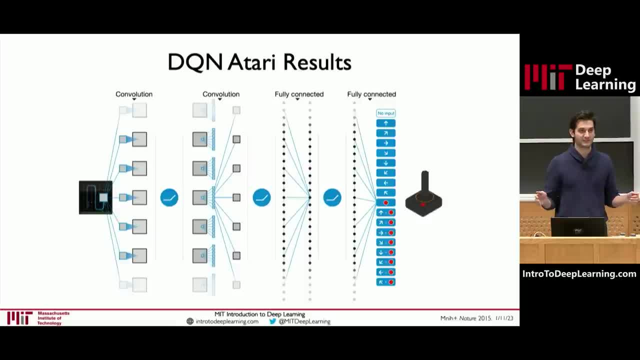 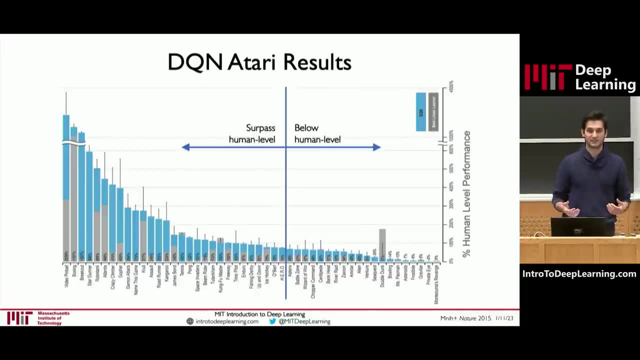 network for a variety of different tasks all across the Atari Breakout ecosystem of games And for each of these tasks, the really fascinating thing that they showed was for this very simple algorithm which really relies on random choice of selection of actions and then learning from. 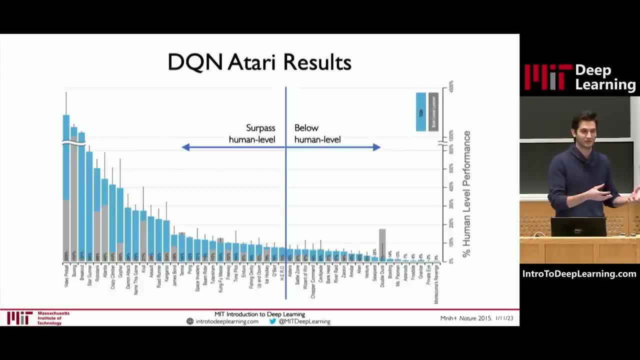 actions that don't do very well, that you discourage them and trying to do actions that did perform well more frequently. So you could train this one network for a variety of different tasks And for each of these tasks, the really fascinating thing that they showed was for this, very simple 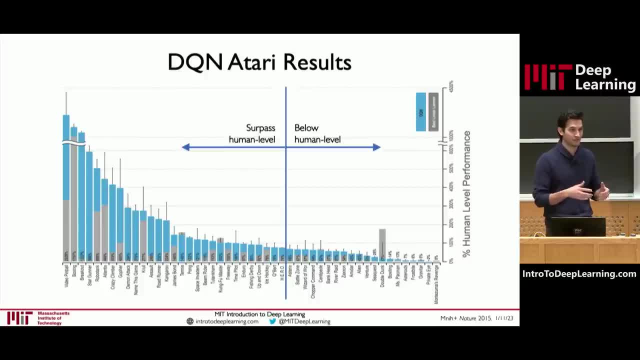 algorithm. but what they found was, even with that type of algorithm, they were able to surpass human level performance on over half of the game. There were some games that you can see here were still below human level performance, but, as we'll see, this was really such an exciting advance because 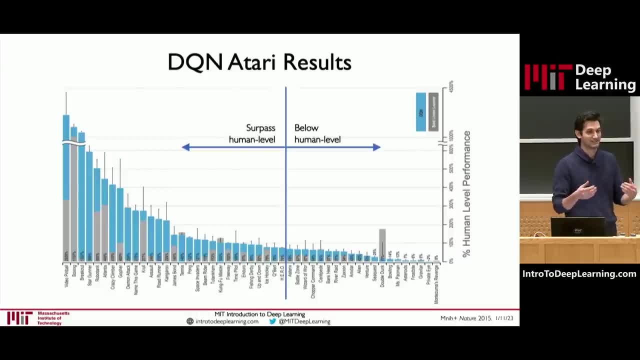 of the simplicity of the algorithm and how clean the formulation of the training was. You only needed a very little amount of prior knowledge to impose onto this neural network for it to be able to learn how to play the game. So this was a very simple algorithm, but what they found was even with 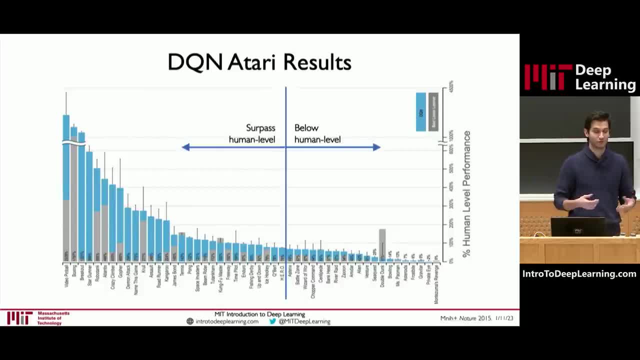 the basic rules. you never had to teach it how to play these games. You never had to teach it any of the rules of the game, right? You only had to let it explore its environment, play the game many, many times against itself and learn directly from that data. Now there are several very important. 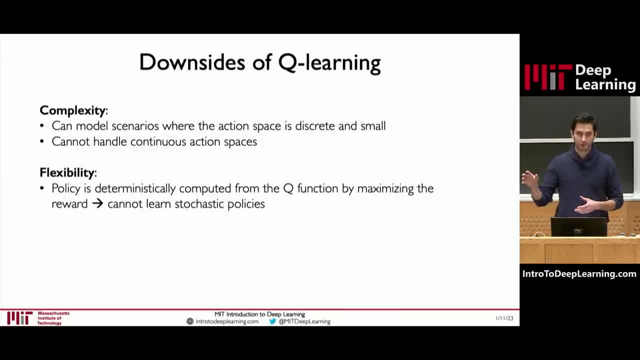 downsides of Q-learning and hopefully these are going to motivate the second part of today's lecture, which we'll talk about. But the first one that I want to really convey to everyone here is that Q-learning is naturally applicable to discrete action spaces. For example, if you have a 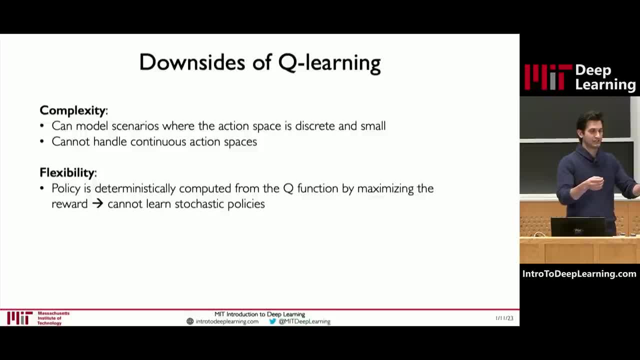 continuous action space. you can think of this output space that we're providing as kind of like one number per action that could be taken. Now, if we have a continuous action space, we have to think about clever ways to work around that. In fact, there are now, more recently there are some. 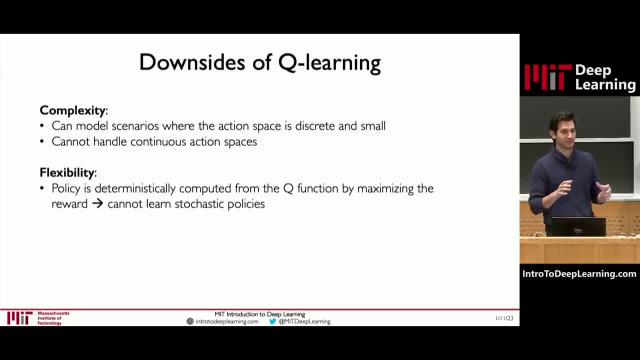 solutions to achieve Q-learning and continuous action spaces, but for the most part Q-learning is very well suited for discrete action spaces and we'll talk about ways of overcoming that with other approaches a bit later. And the second component here is that the policy that we're learning right- the Q function- is giving rise to that policy. 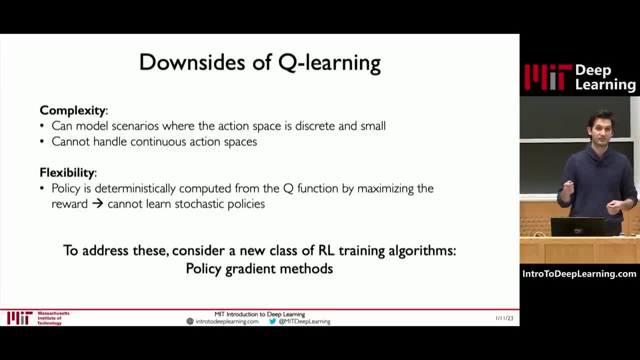 which is the thing that we're actually using to determine what action to take, given any state. That policy is determined by, you know, deterministically, optimizing that Q function. We simply look at the results from the Q function and apply our or we look at the results of the Q. 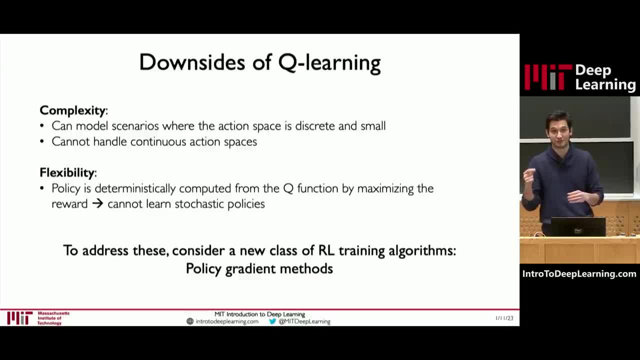 function and we pick the action that has the best or the highest Q value. That is very dangerous in many cases because of the fact that it's always going to pick the best value for a given state. There's no stochasticity in that pipeline, so you can. 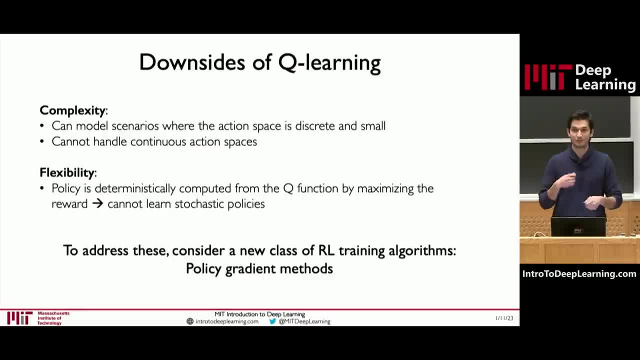 very frequently get caught in situations where you keep repeating the same actions and you don't learn to explore potentially different options that you may be thinking of So to address these very important challenges. that's hopefully going to motivate now the next part of today's lecture. 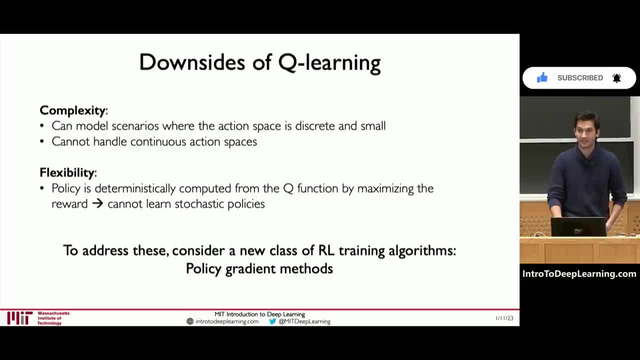 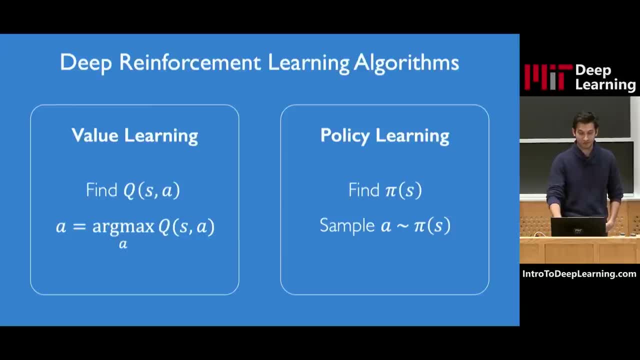 which is going to be focused on policy learning, which is a different class of reinforcement learning algorithms that are different than Q learning algorithms And, like I said, those are called policy gradient algorithms. In policy gradient algorithms, the main difference is that, instead of trying to infer the policy from, 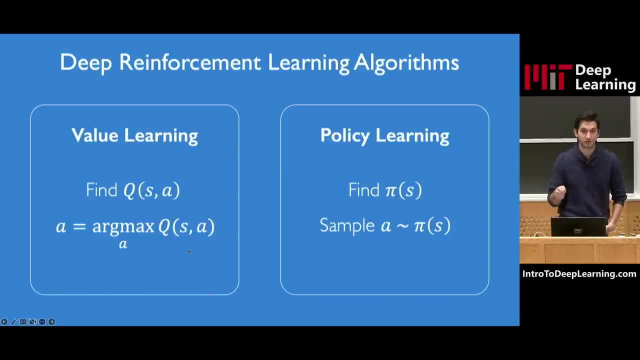 the Q function. we're just going to build a neural network that will directly learn that policy function from the data right. So it kind of skips one step and we'll see how we can train those networks. So before we get there, let me just review. 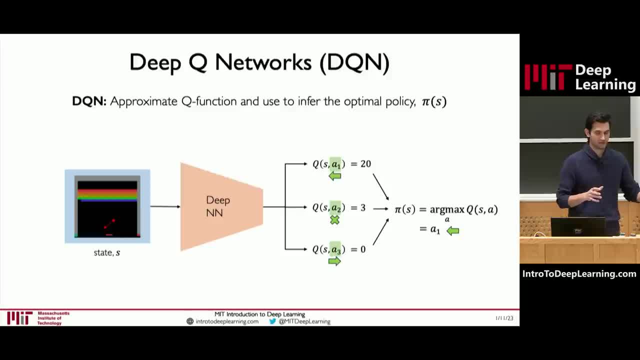 Let's revisit one more time the Q function illustration that we are looking at. right Q function- we are trying to build a neural network- outputs these Q values- one value per action- and we determine the policy by looking over this state of Q values, picking the value that has the 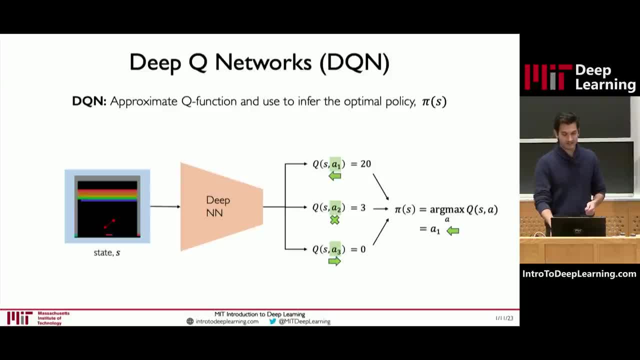 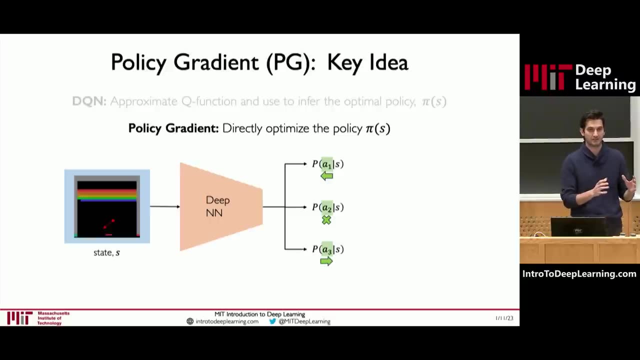 highest and looking at its corresponding action Now with policy networks. the idea that we want to keep here is that instead of predicting the Q values themselves, let's directly try to optimize the policy function. Here we're calling the policy function pi of s right, So pi is the policy. 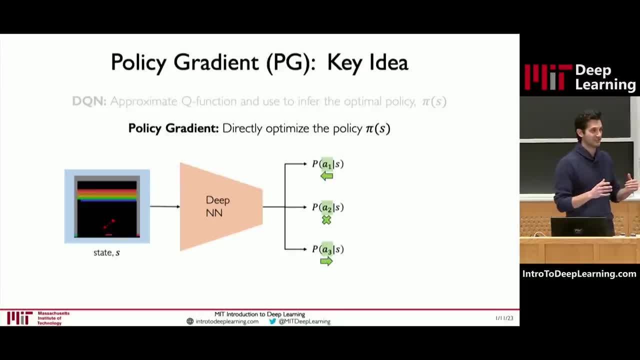 s is our state. So it's a function that takes as input only the state and it's going to directly output the action. So the outputs here give us the desired action that we should take in any given state that we find ourselves in, And that represents not only the best action. 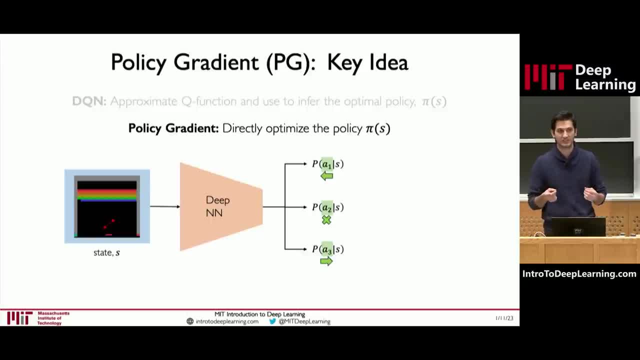 that we should take, but let's denote this as basically the probability that selecting that action would result in the output And a very desirable outcome for our network. So not necessarily the value of that action, but rather the probability that selecting that action would be the highest value, right? So 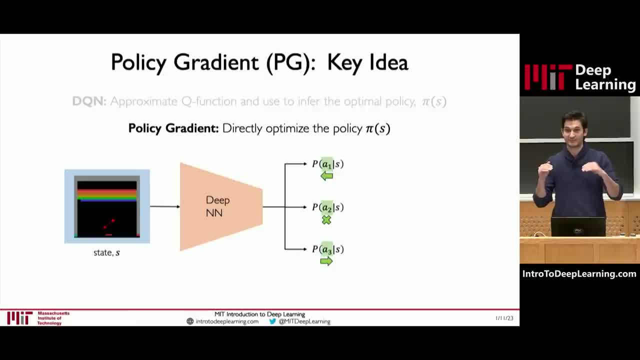 you don't care exactly about what is the numerical value that selecting this action takes or gives rise to, rather, but rather what is the likelihood that selecting this action will give you the best performing value that you could expect Exactly. In fact, value itself doesn't matter. You only care about if selecting this action 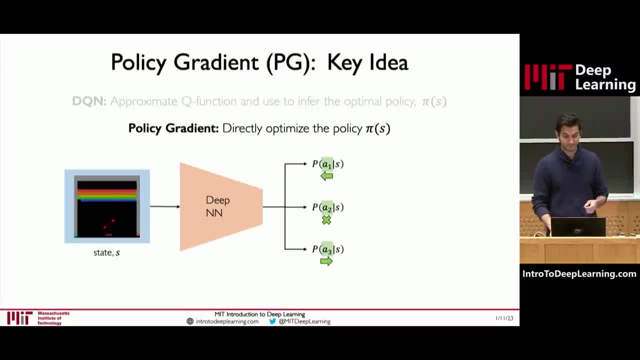 is going to give you, with high likelihood, the best one. So we can see that if these predicted probabilities here right in this example of Atari right, going left has the probability of being the highest value action with 90% staying in the center, that's a probability of 10%, and going right is 0%. 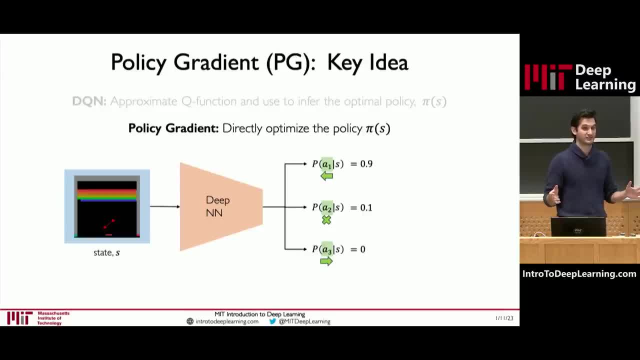 So, ideally, what our neural network should do in this case is, 90% of the time in this situation, go to the left. 10% of the time it could still try staying where it is, but never it should go to the right. Now, note that this now is a probability distribution. This is very different. 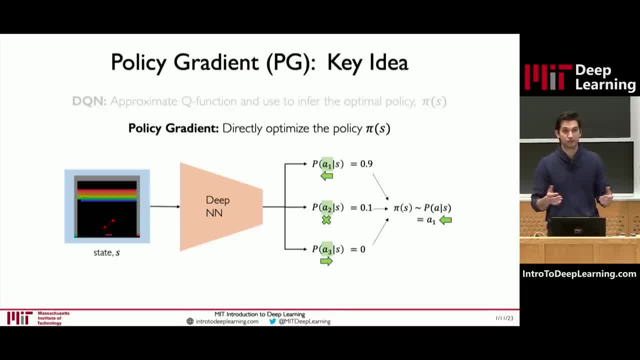 than a Q function. A Q function has actually no structure right. The Q values themselves can take any real number, right. But here the policy network has a very formulated output. All of the numbers here in the output have to sum to one, because this is a probability distribution. 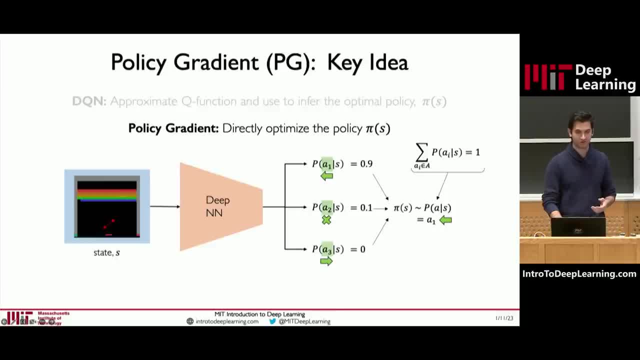 right And that gives it a very rigorous version of how we can train this model. that makes it a bit easier to train than Q functions as well. So one other very important advantage of having an output that is, a probability distribution is actually going to tie back to this other issue. 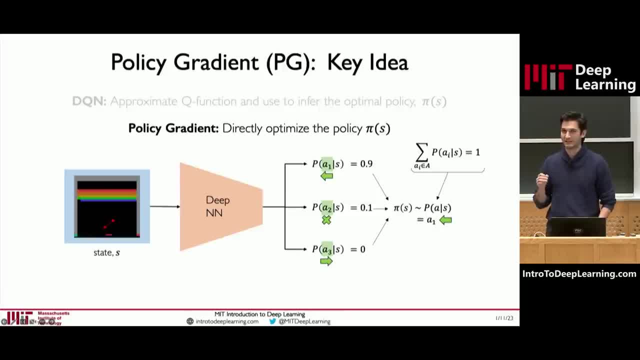 of Q functions and Q neural networks. So let's take a look at the next slide. So the first thing we want to do is take a look at what we're doing with this network and look at how we're pathogenizing affects this dynamicAM over the time. remedy: internallβ. 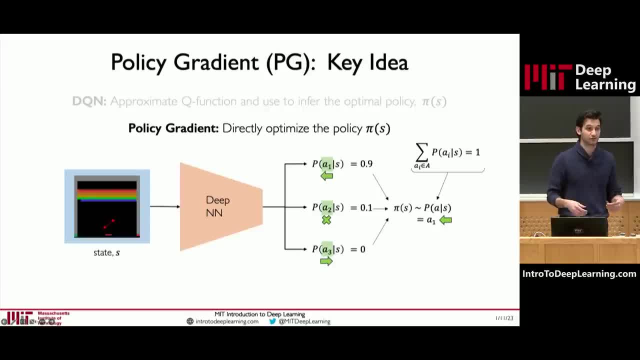 currently incomplete. So within this meta- intervals, we'll compare some of the species of neural networks that we saw before, And that is the fact that Q functions are naturally suited towards discrete action spaces. Now, when we're looking at this policy network, we're outputting a distribution. 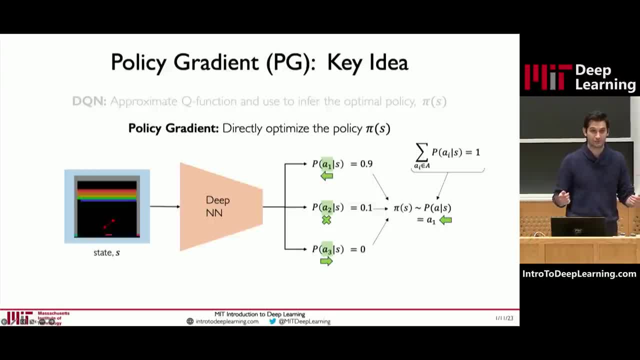 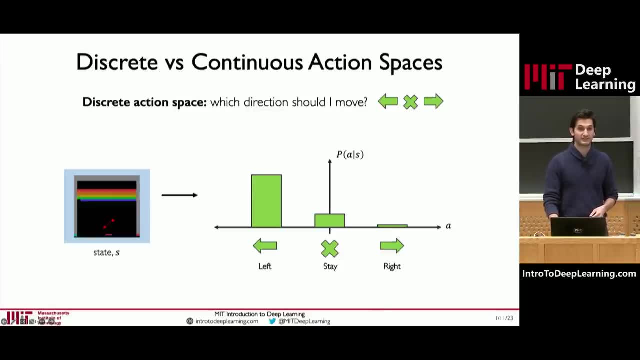 how we could learn to predict uncertainties, which are continuous probability distributions, using data. And just like that, we could also use this same formulation to move beyond discrete action spaces, like you can see here, which are one possible action, a probability associated to one possible action, in a discrete set of possible actions. Now we may have a space. 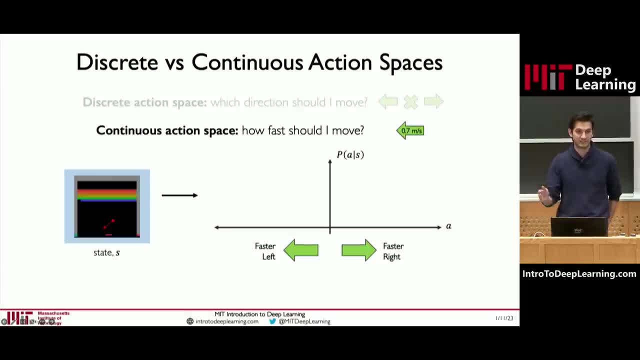 which is not what action should I take- go left, right or stay in the center- but rather how quickly should I move and in what direction should I move right? That is a continuous variable as opposed to a discrete variable, And you could say that now the answer should look like this: right Moving. 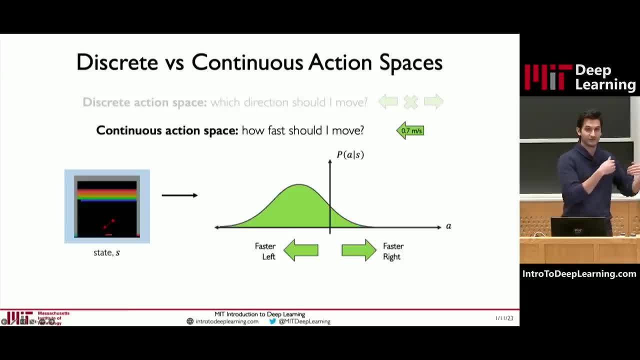 very fast to the right versus very slow to the or, excuse me, very fast to the left versus very slow to the left, has this continuous spectrum that we may want to model. Now, when we plot this entire distribution of taking an action, giving a state, you can see basically a very simple illustration of that right here. This: 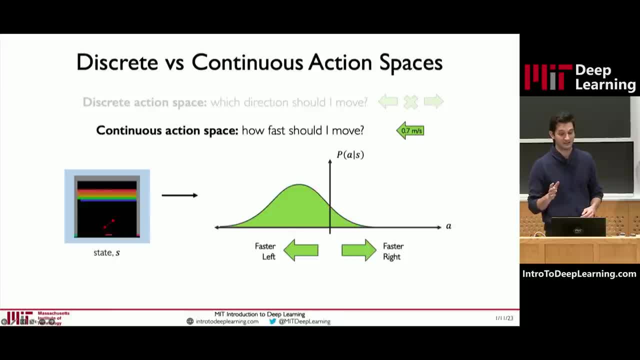 distribution has most of its mass over- or sorry, it has all of its mass over the entire real number line. first of all, It has most of its mass right in the optimal action space that we want to take. So if we want to determine the best action to take, we would simply take the mode of this. 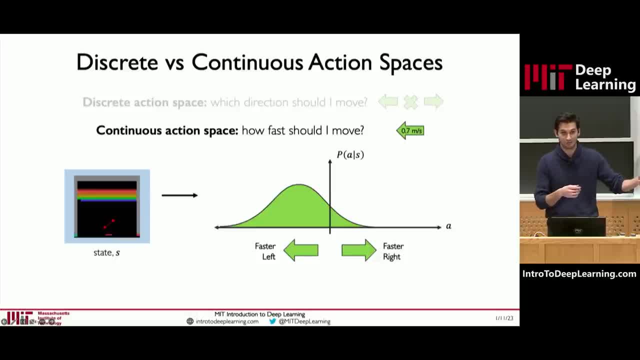 distribution right, the highest point, That would be the speed at which we should move and the direction that we should move in. So if we want to determine the best action to take, we would simply take the mode of this distribution right. So if we wanted to also, you know, try out different things and explore our 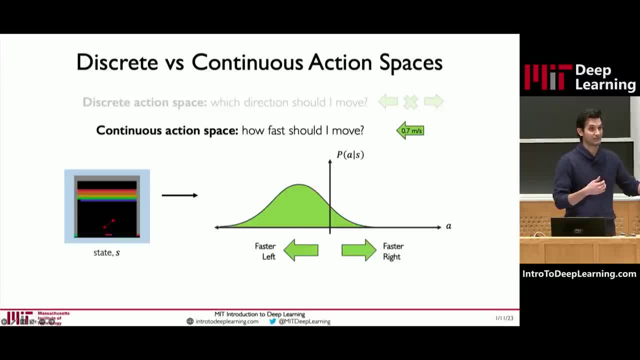 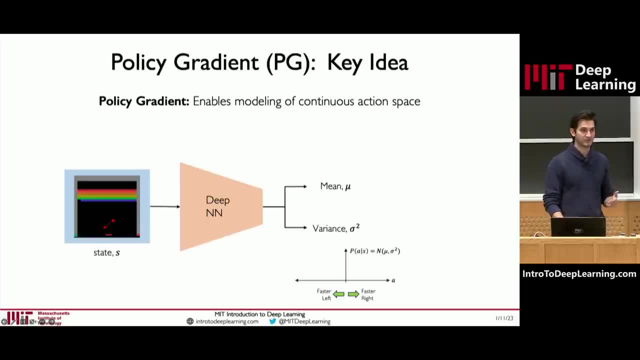 space we could sample from this distribution and still obtain some stochasticity. Now let's look at an example of how we can actually model these continuous distributions, And actually we've already seen some examples of this in the previous two lectures, like I. 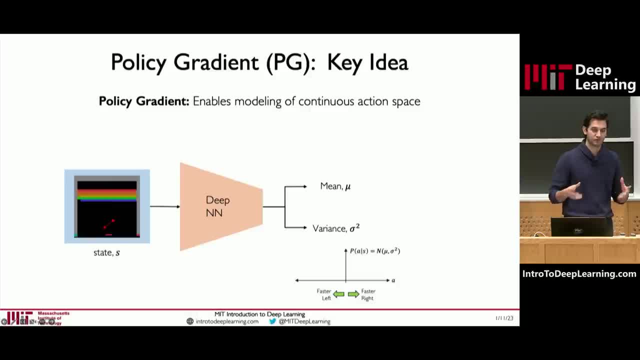 mentioned, But let's take a look specifically in the context of reinforcement learning and policy gradient learning. So, instead of predicting this probability of taking an action, giving all possible states- which in this case, there is now an infinite number of because we're in the 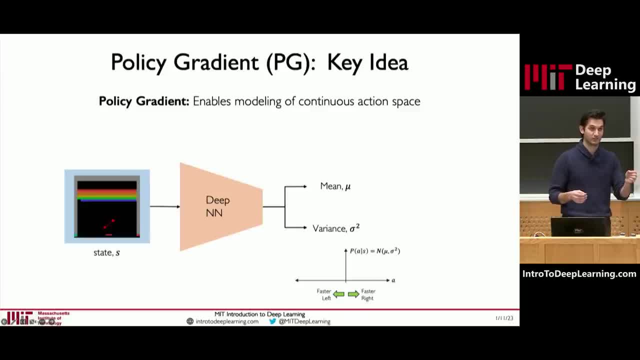 continuous domain, we can't simply predict a single probability for every possible action, because there is an infinite number of them. So instead, what if we parametrized our action space by a distribution right? So let's take, for example, the Gaussian distribution To parametrize a. 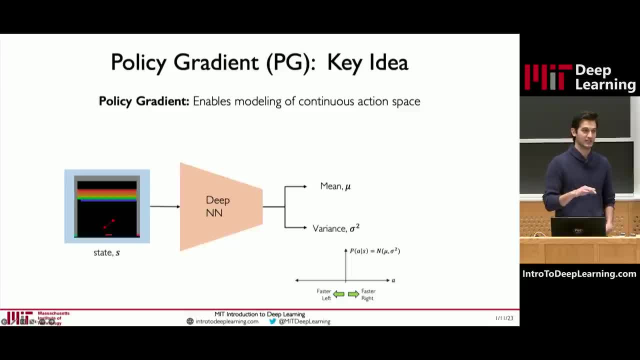 Gaussian distribution. we only need two outputs, right, We need a mean and a variance. Given a mean and a variance, we can actually have a probability mass and we can compute a probability over any possible action that we may want to take, just from those two numbers. So, for example, in this image here we may: 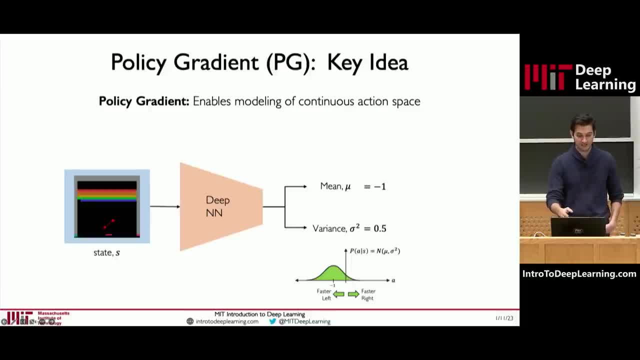 want to output a Gaussian that looks like this: right its mean is centered at- let's see- negative 0.8, indicating that we should move basically left with a speed of 0.8 meters per second, for example. and again, we can see that because this is a probability distribution, because of the format, 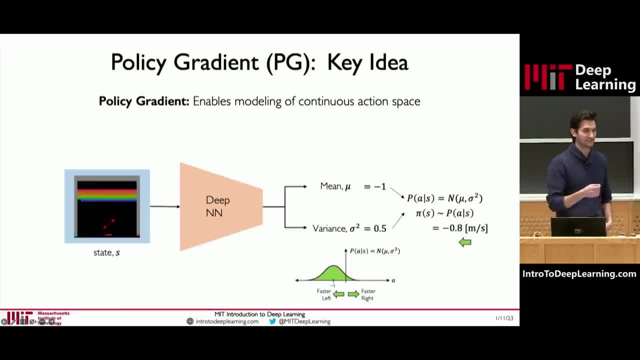 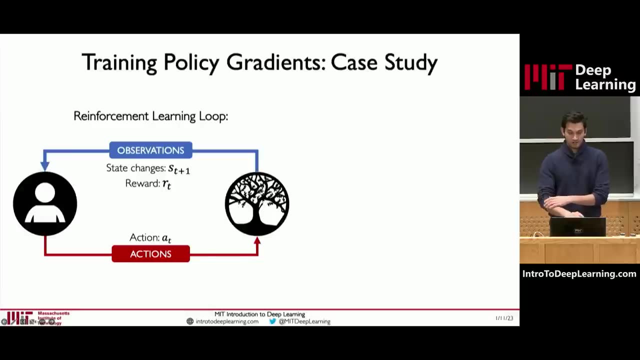 of policy networks. right, we're enforcing that this is a probability distribution. that means that the integral now of this, of these outputs- right by definition of it being a Gaussian- must also integrate to one. Okay, great. so now let's maybe take a look at how policy gradient networks 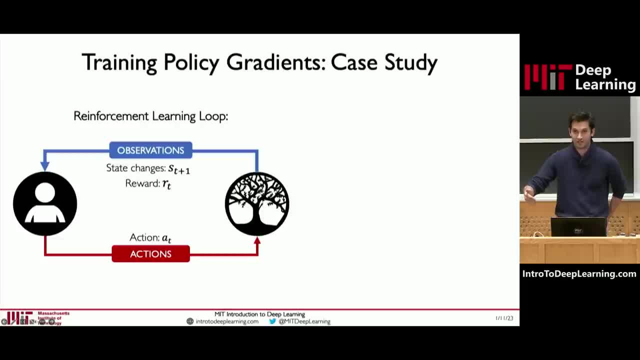 can be used to integrate, Can be trained and, you know, step through that process as well. as we look at a very concrete example, and maybe let's start by just revisiting this reinforcement learning loop that we started this class with. Now let's specifically consider the example of training an autonomous vehicle. 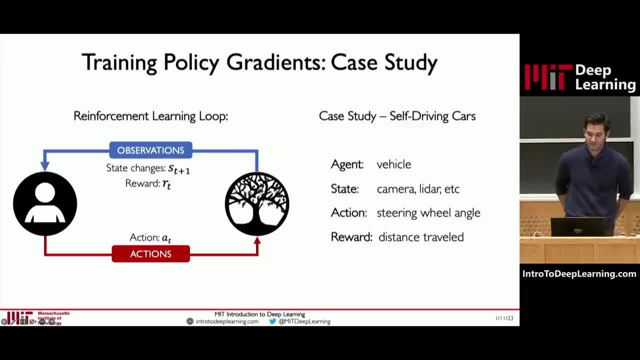 since I think that this is a particularly, very intuitive example that we can walk through. The agent here is the vehicle right. the state could be obtained through many sensors that could be mounted on the vehicle itself. so, for example, autonomous vehicles are typically equipped with sensors like cameras, lidars, radars, etc. All of these are giving observational inputs to the 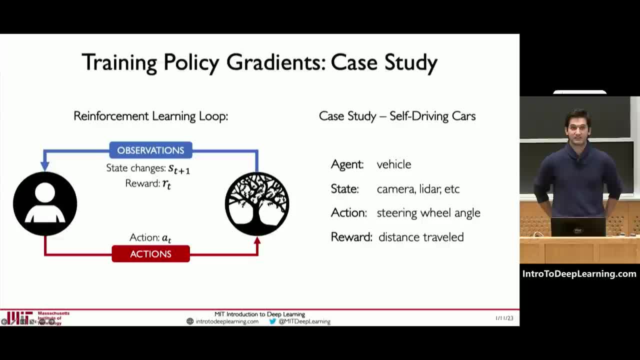 to the vehicle. The action that we could take is a steering wheel angle. this is not a discrete variable, this is a continuous variable. it's actually an angle that could take any real number. and finally, the reward in this very simplistic example is the distance that we travel before we 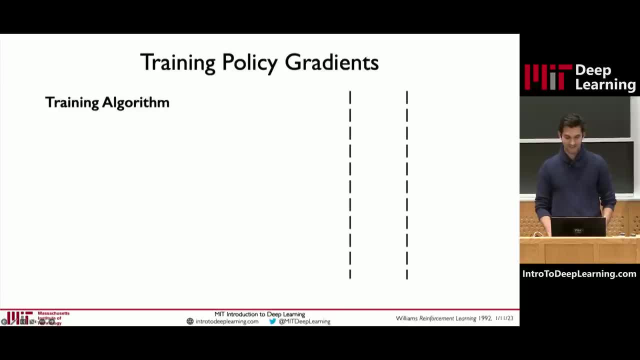 crash. Okay. so now let's take a look at how we could train a policy gradient neural network to solve this task of self driving cars as a concrete example. So we start by initializing our agent, right? remember that we have no training data, right. so we have to think about actually reinforcement. learning is almost like a data acquisition plus learning pipeline combined together. so the first part of that data acquisition pipeline is first to initialize our agent to go out and collect some data. 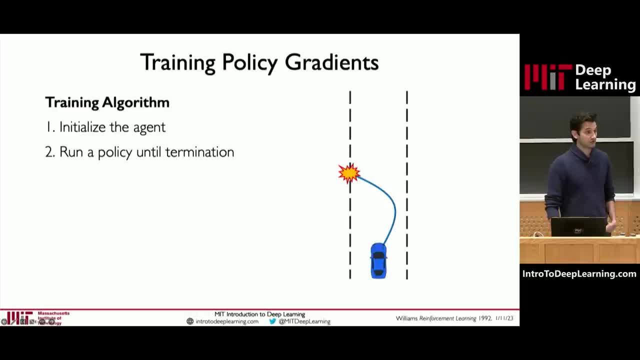 So we start our Vehicle, our agent, and in the beginning, of course, it knows nothing about driving. it's never been exposed to any of these rules of the environment or the observation before, so it runs its policy, which right now is untrained entirely. 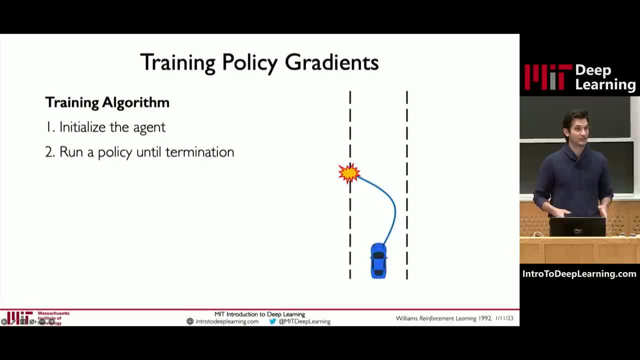 Until it terminates, right until it goes outside of some bounds that we define. we measure basically the reward as the distance that you traveled before it terminated And we record All of the states, all of the states that we travel to, and the distance that we travel to and we recodie all of the states that we travel to. we recodie all of the states that we travel to. 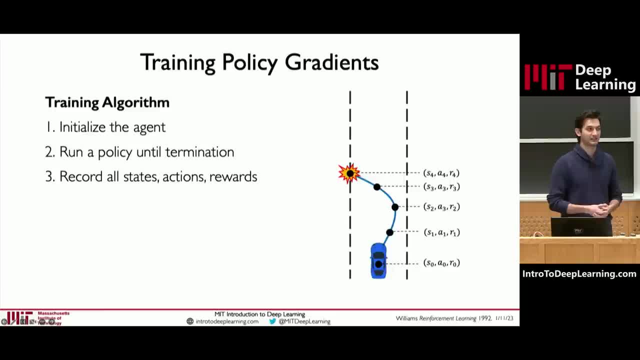 All of the states that we travel to, of the actions and the final reward that it obtained until that termination. This becomes our mini data set that we'll use for the first round of training. Let's take those data sets and now we'll do one step of training. 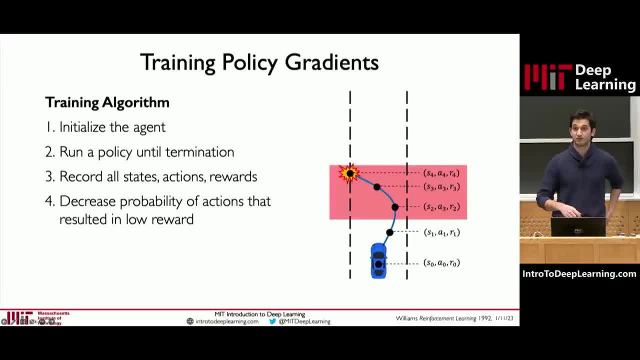 The first step of training that we'll do is to take the later half of our trajectory that our agent ran and decrease the probability of actions that resulted in low rewards. Because we know the vehicle terminated, we can assume that all of the actions that occurred. 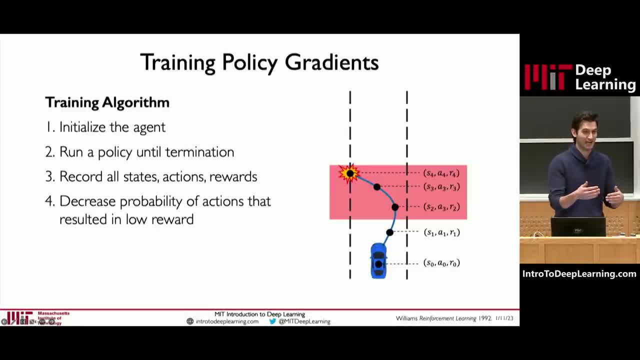 in the later half of this trajectory were probably not very good actions because they came very close to termination. Let's decrease the probability of all of those things happening again in the future. We'll take all of the things that happened in the beginning half of our training episode. 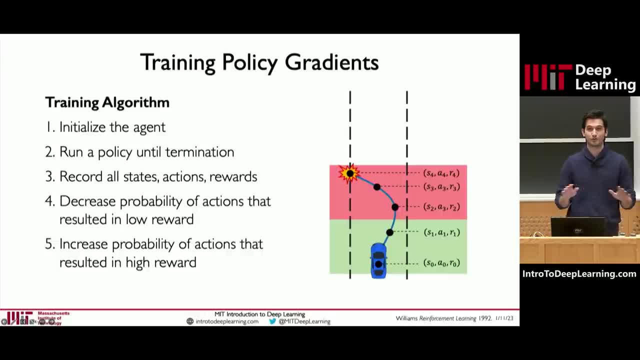 and we will increase their probability. Now again, there's no reason why there shouldn't necessarily be a good action that we took in the first half of this trajectory and a bad action in the later half, but it's simply because actions that are in the later half were closer to a failure and closer to termination. 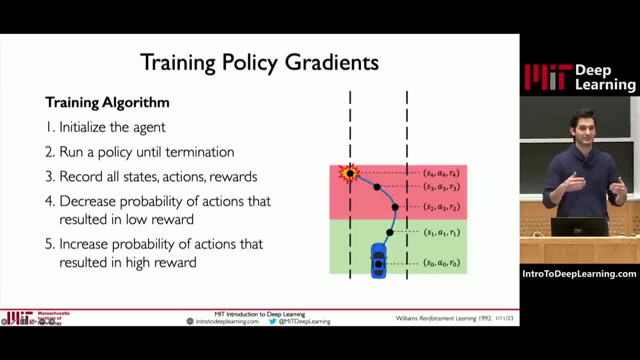 that we can assume, for example, that these were probably suboptimal actions, but it's very possible that these are noisy rewards as well, because it's such a sparse signal, It's very possible that you had some good actions at the end. 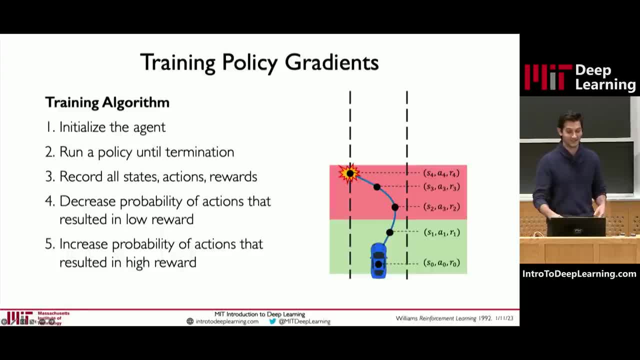 You were actually trying to recover your car, but you were just too late. Now repeat this process again, Reinitialize the agent one more time and run it until completion. Now the agent goes a bit farther because you've decreased the probabilities at the end increased. 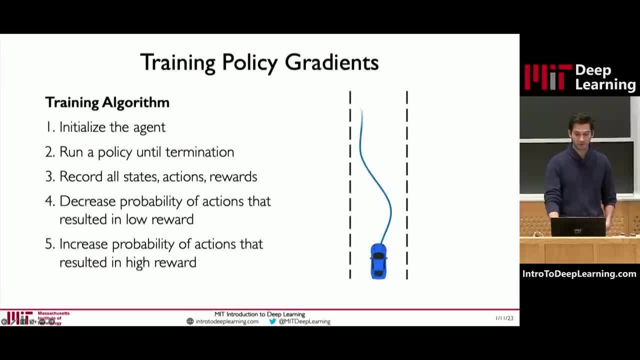 the probabilities at the future, and you keep repeating this over and over again until you notice that the agent learns to perform better and better every time until it finally converges At the end. the agent is able to basically follow lanes, usually swerving a bit side to side, while it does that without crashing. 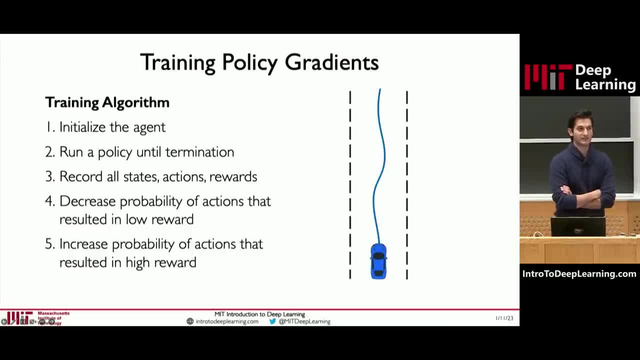 and this is actually really fascinating because this is a self-driving car that we never taught anything about what a lane marker means or what are the rules of the road, anything about that right, this was a car that learned entirely just by going out, crashing a lot and, you know, trying. 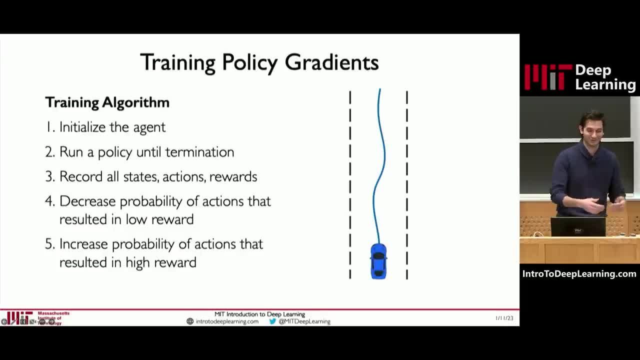 to figure out what to do to not keep doing that in the future. right, and the remaining question is actually how we can update, you know, that policy as part of this algorithm that i'm showing you on the right and the left hand side. right, like: how can we basically formulate that same algorithm? 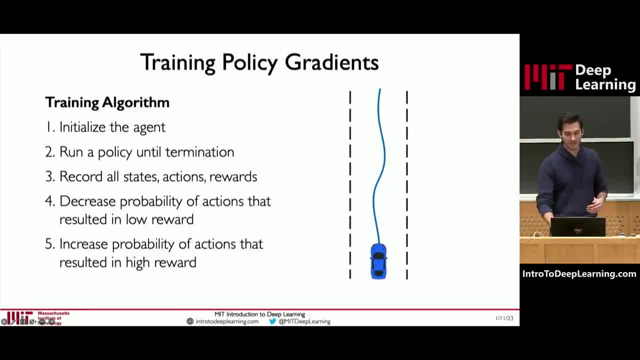 and specifically the update equation, steps four and five. right here, these are the two really important steps right of how we can use those two steps to train our policy and decrease the probability of bad events while promoting these likelihoods of all these good events. so let's assume the let let's. 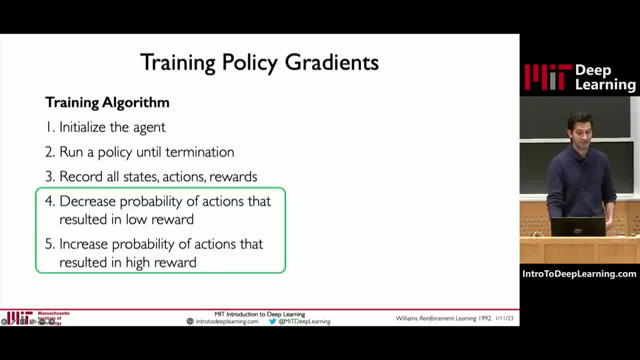 look at the loss function first of all. the loss function for a policy gradient neural network looks like this, and then we'll start by dissecting it to understand why this works the way it does. so here we can see that the loss consists of two terms. the first term is this term in green. 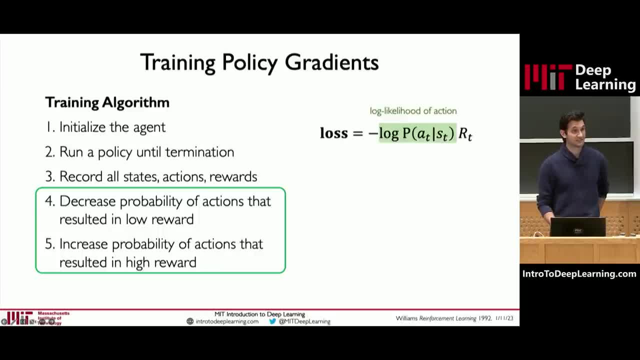 which is called the log likelihood of selecting a particular action. the second term is something that all of you are very familiar with already. this is simply the return at a specific time, right? so that's the expected return on rewards that you would get after this time point. now, let's assume that we 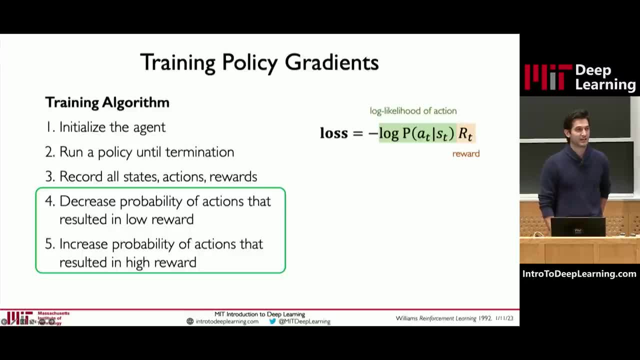 got a lot of reward for a particular action that had a high log probability or a high probability. right, if we got a lot of reward for a particular action that had high probability, that means that we want to increase that probability even further. so we do it even more, or even more likelihood. we 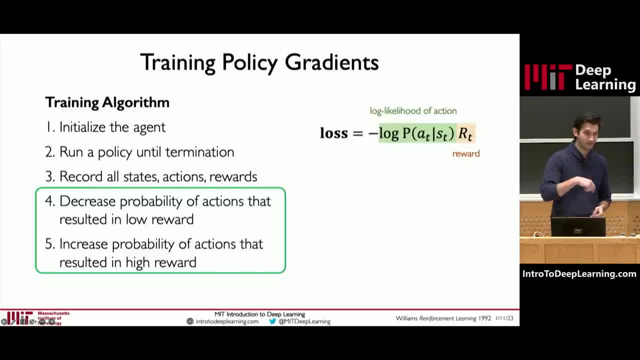 sampled that action again into the future. on the other hand, if we collected, or let's say, if we obtained a reward that was very low for an action that had high likelihood, we want the inverse effect, right. we never want to sample that action again in the future because it resulted in a low reward. right, and you'll notice that this loss function right. 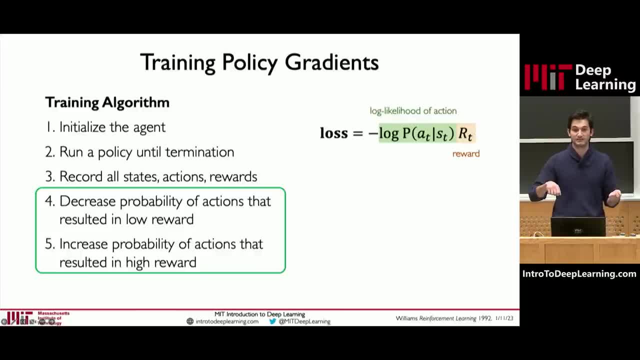 here. by including this negative, we're going to minimize the likelihood of achieving any action that had low rewards in this trajectory. now, in our simplified example on the car example, all the things that had low rewards were exactly those actions that came closest to the termination part of the neural of the vehicle right. all the things that had high rewards were. 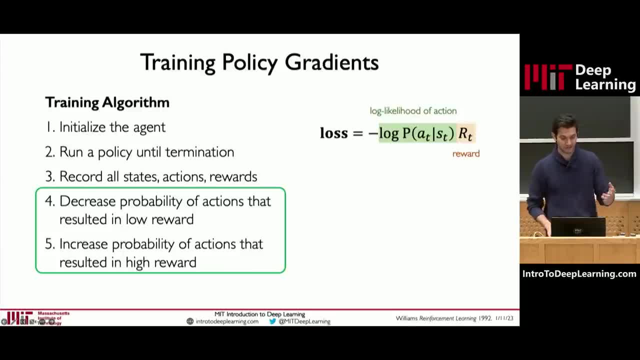 the things that came in the beginning. that's just the assumption that we make when defining our reward structure. now we can plug this into the the loss of gradient descent algorithm to train our neural network when we see, you know this policy, gradient algorithm, which you can see highlighted. 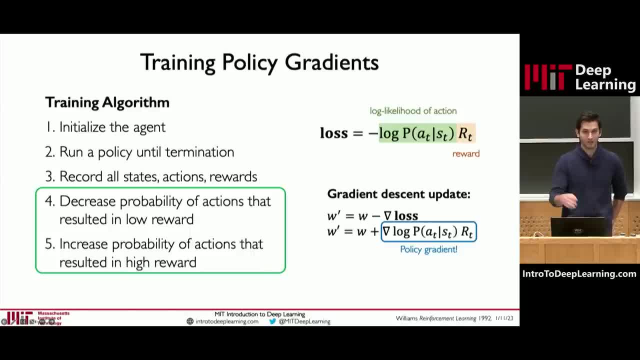 here. this gradient is exactly of the policy part of the neural network. that's the probability of selecting an action given a specific state, and if you remember before when we defined, you know what does it mean to be a policy function. that's exactly what it means, right given a particular state that you 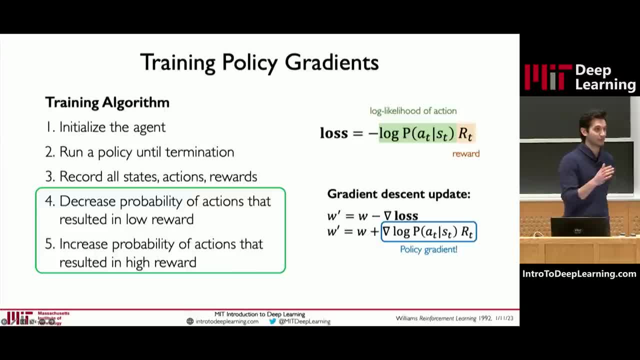 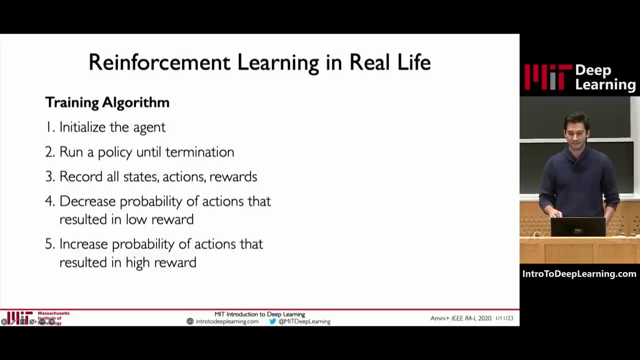 find yourself in: what is the probability of selecting a particular action with the highest likelihood, and that's you know exactly where this method gets its name from, this policy gradient piece here that you can see here. now I want to take maybe just a very brief second towards the end of the class here just to talk about 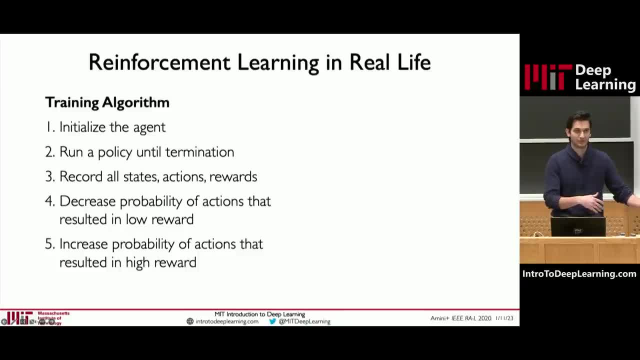 you know some of the the challenges and, keeping in line with the first lecture today, some of the challenges of deploying these types of algorithms in the context of the real world. right, what do you think when you look at this training algorithm that you can see here? right, what do you think? 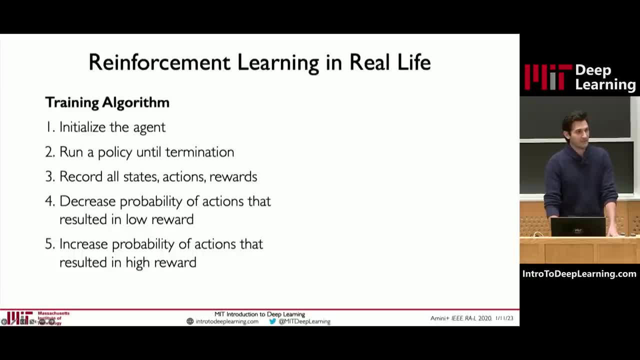 are the shortcomings of this training algorithm and which step I guess specifically if we wanted to deploy this approach into reality. Yeah, exactly, So it's step two, right, If you wanted to do this in reality, right, that essentially means that you want to go out collect your car, crashing it a bunch of 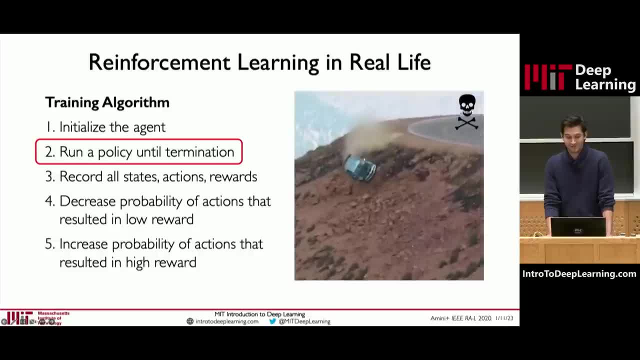 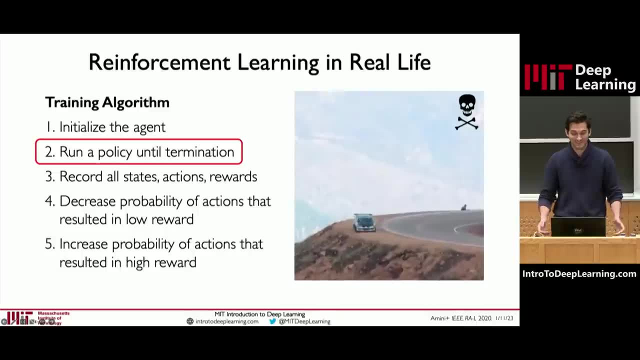 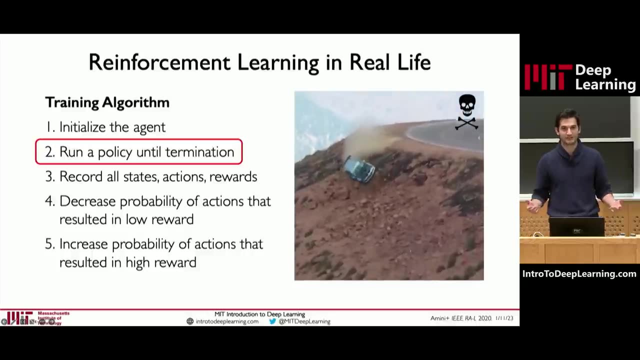 times just to learn how to not crash it right, And that's, you know, that's simply not feasible, right Number one: It's also, you know, very dangerous number two. So there are ways around this. right, The number one way around this is that people try to train these types of models. 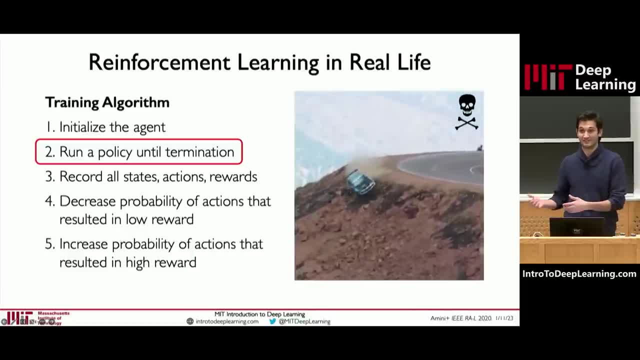 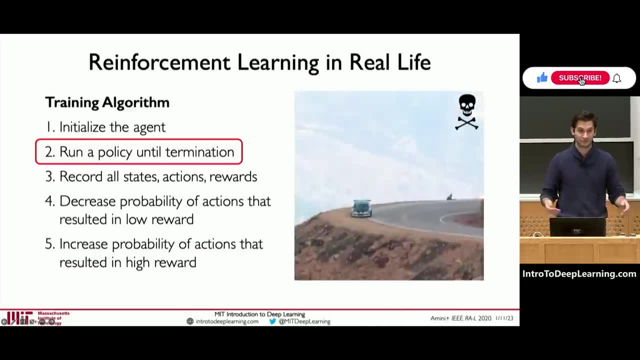 in simulation. right, Simulation is very safe because you know we're not going to actually be damaging anything real. It's still very inefficient because we have to run these algorithms a bunch of times and crash them a bunch of times just to learn how not to crash. 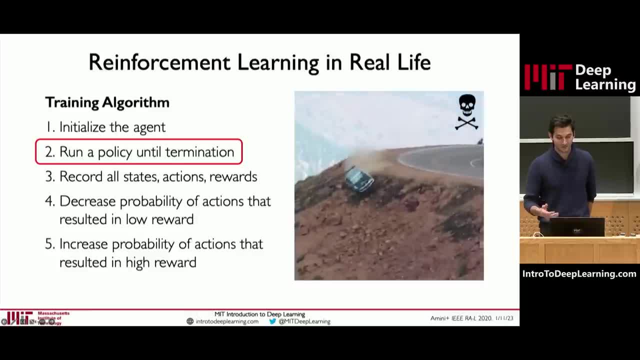 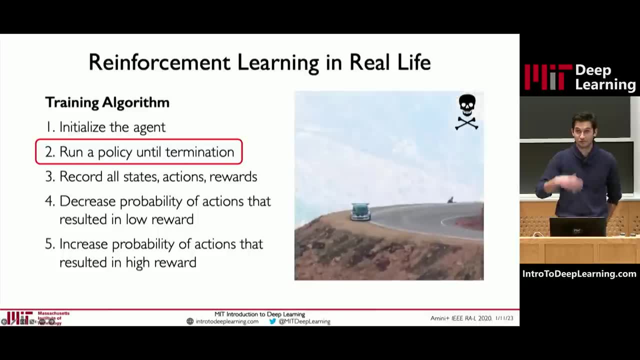 But at least now, at least from a safety point of view, it's much safer. But you know, the problem is that modern simulation engines for reinforcement learning and generally, very broadly speaking, modern simulators for vision specifically do not at all. 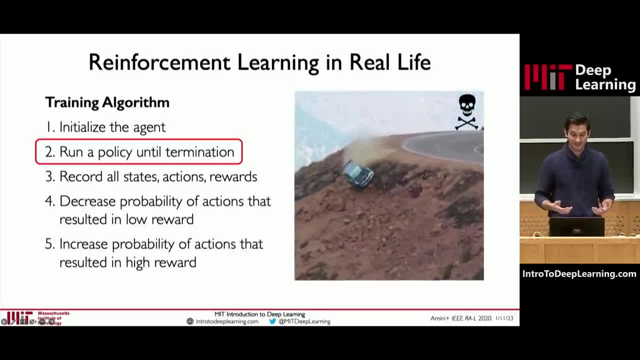 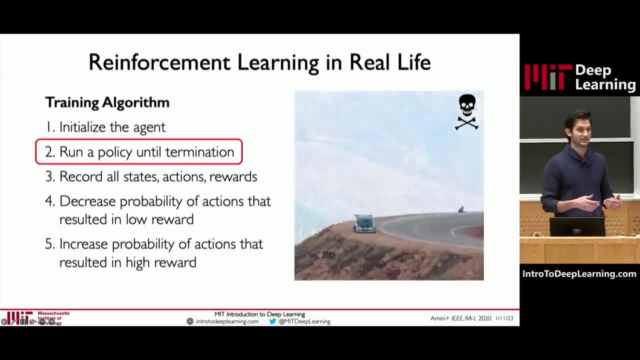 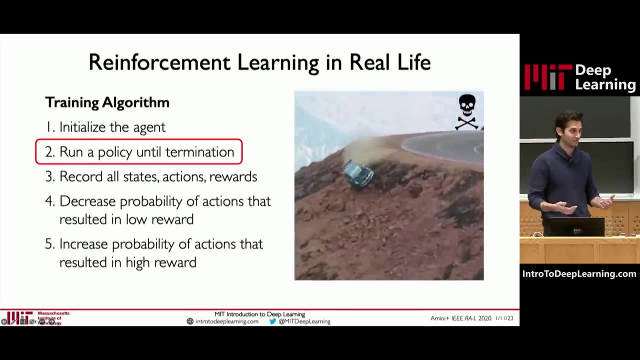 capture reality very accurately. In fact, there's a very famous notion called the sim-to-real gap, which is a gap that exists when you train algorithms in simulation, and they don't extend to a lot of the phenomena that we see and the patterns that we see in reality, And one really. 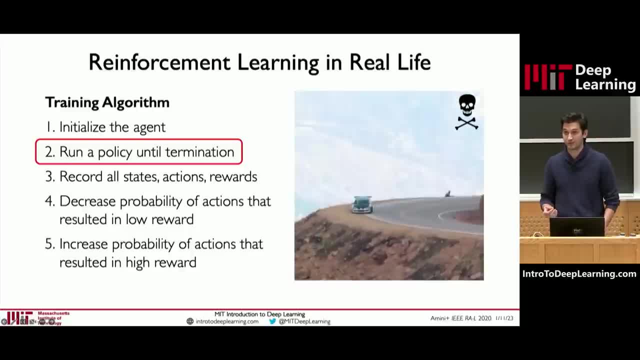 cool result that I want to just highlight here is that when we're training reinforcement learning algorithms, we ultimately want them to be, you know, not operating in simulation, We want them to be in reality And as part of our lab here at MIT. 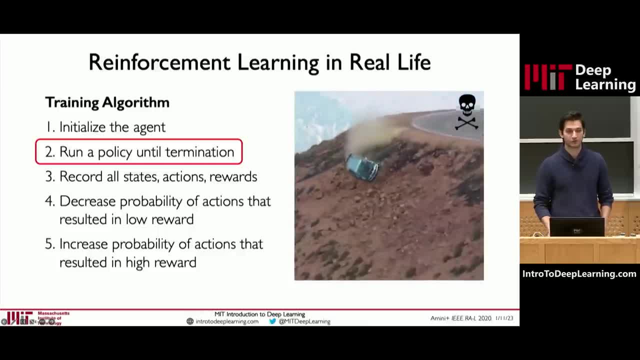 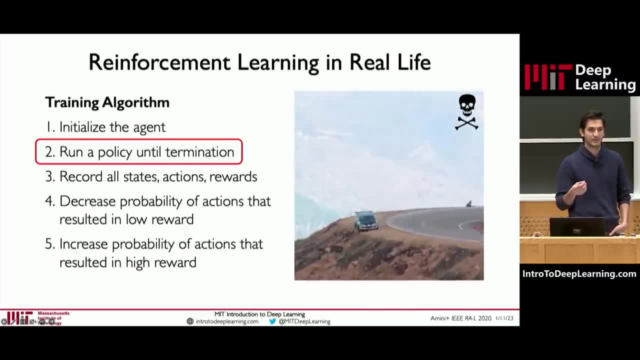 we've been developing this very, very cool brand new photorealistic simulation engine that goes beyond basically the paradigm of how simulators work today, which is basically defining a model of their environment and trying to, you know, synthesize that model. Essentially, these: 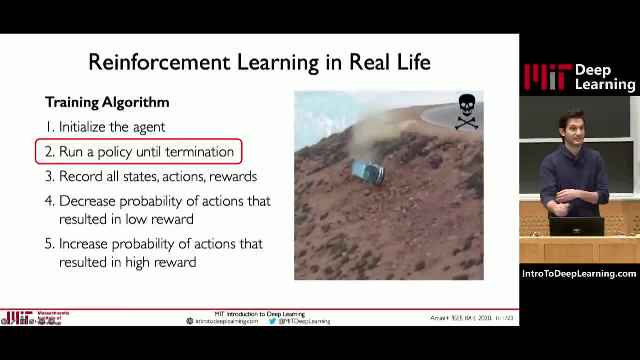 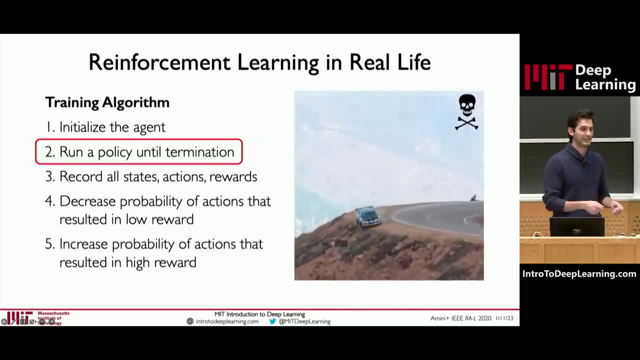 simulators are like glorified game engines, And so you know, we've been trying to, you know, make them look very realistic, right? They all look very game-like when you look at them. But one thing that we've done is taken a data-driven approach. Using real data of the real world can 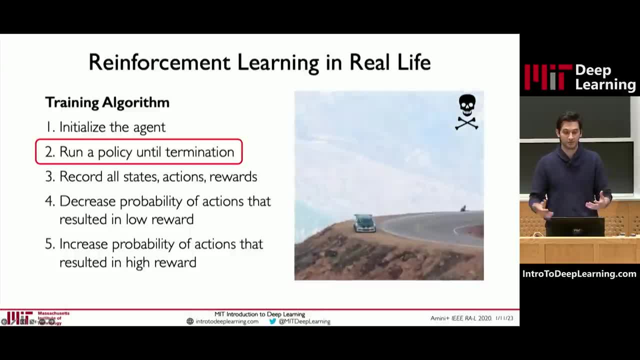 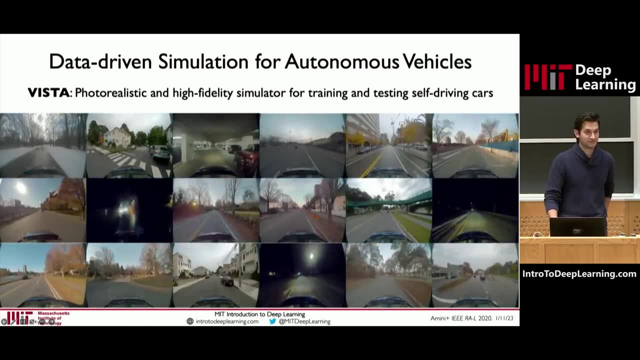 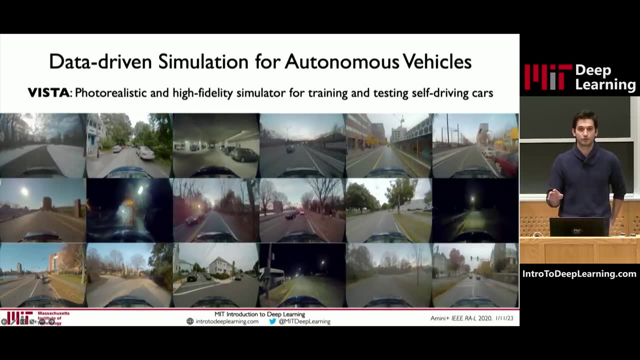 we build up synthetic environments that are super photorealistic and look like this right, So this is a cool result that we created here at MIT, developing this photorealistic simulation engine. This is actually an autonomous agent- not a real car- driving through our virtual simulator in a. 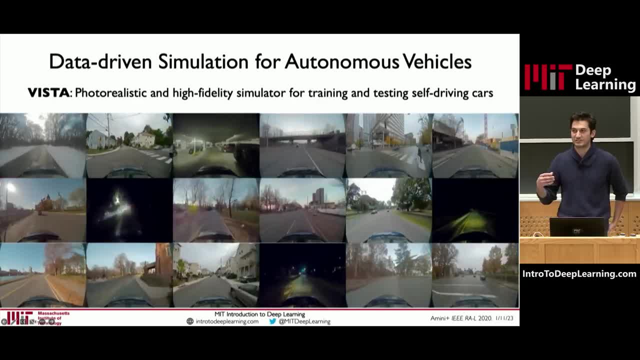 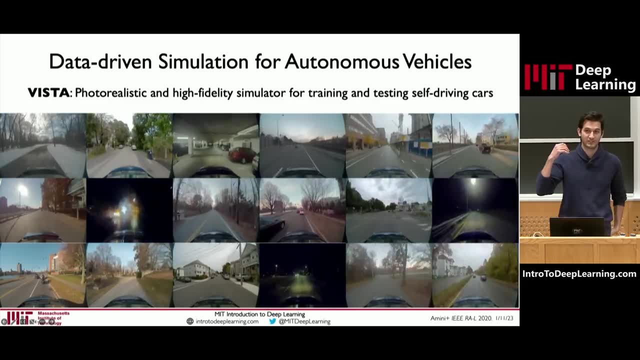 virtual environment And this is a vision of a virtual environment. This is the image that we can use to simulate different scenarios. So this simulator is called Vista. It allows us to basically use real data that we do collect in the real world, but then re-simulate those same. 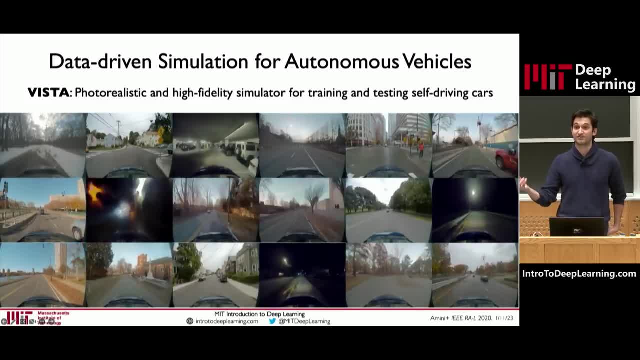 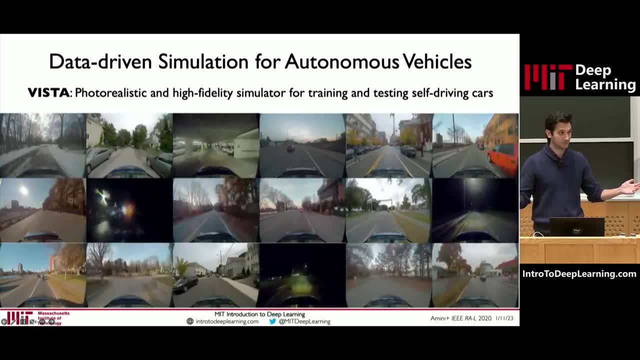 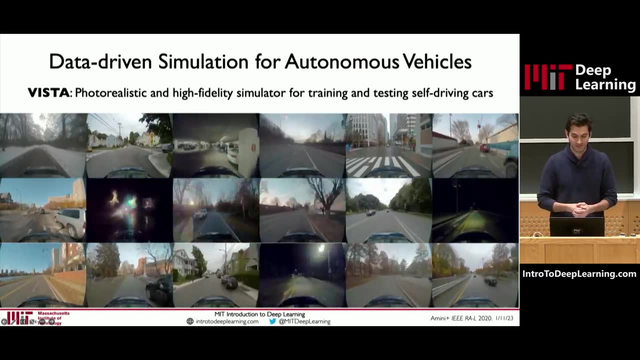 real roads, For example. let's say you take your car, you drive out on Mass Ave, you collect data of Mass Ave. You can now drop a virtual agent into that same simulated environment, observing new perturbations or types of angles that it might be exposed to, And that allows us to train these. 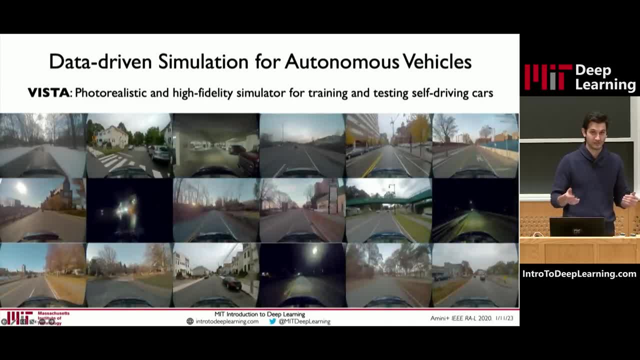 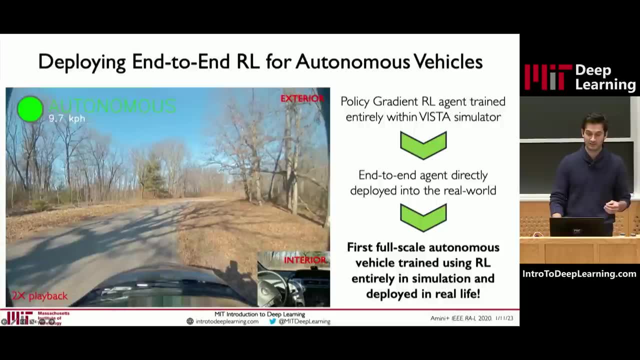 agents, now entirely using reinforcement learning, no human labels, but, importantly, allow them to be transferred into reality, because there's no sim to real gap anymore. So, in fact, we did exactly this: We placed agents into our simulator, We trained them using the exact algorithms that you 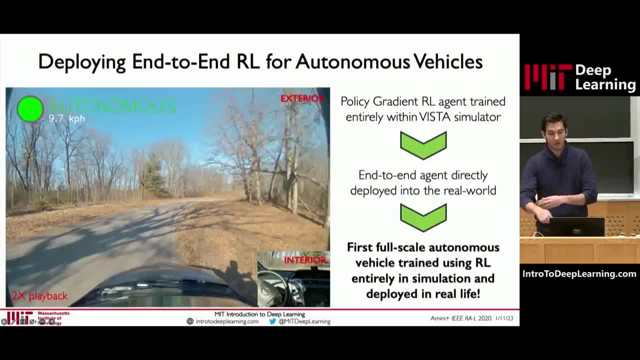 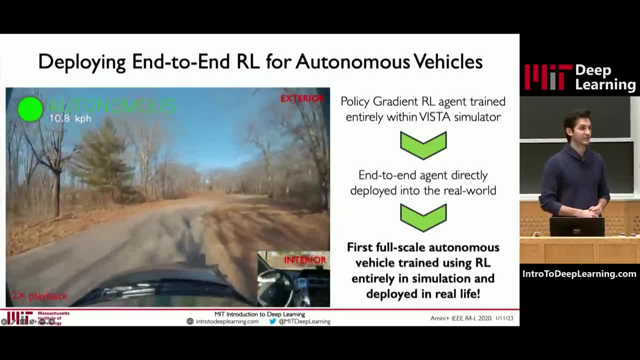 learned about in today's lecture- these policy, gradient algorithms and all of the training was done entirely in simulation. Then we took these policies and we deployed them on board our full scale autonomous vehicle. This is now in the real world, no longer in simulation And on the left. 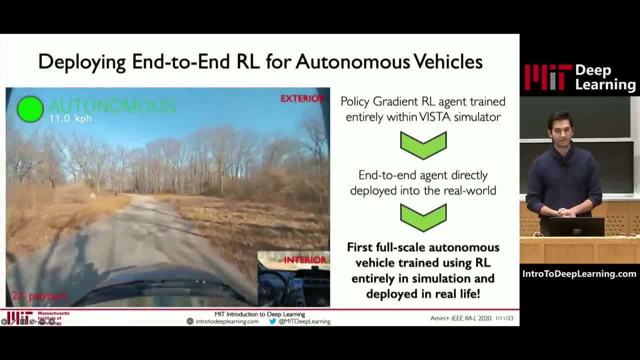 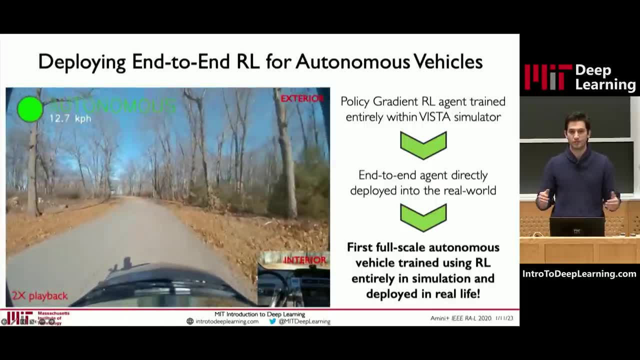 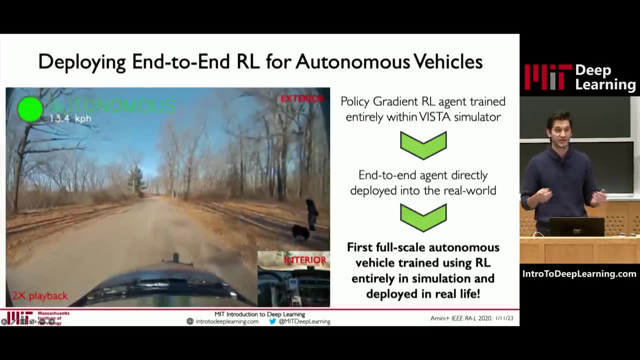 hand side, you can see basically this car driving through this environment completely autonomous in the real world. No transfer learning is done here. There is no augmentation of data from real world data. This is entirely trained using simulation And this represented actually the first time ever that reinforcement. 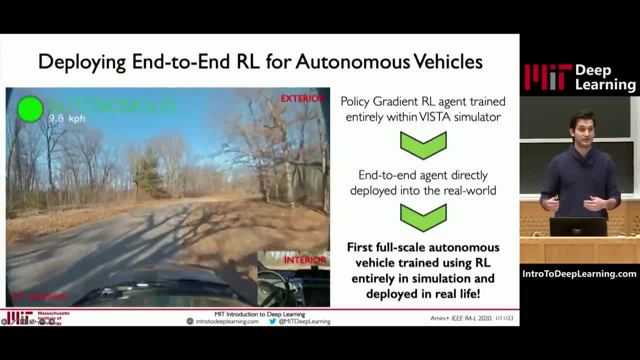 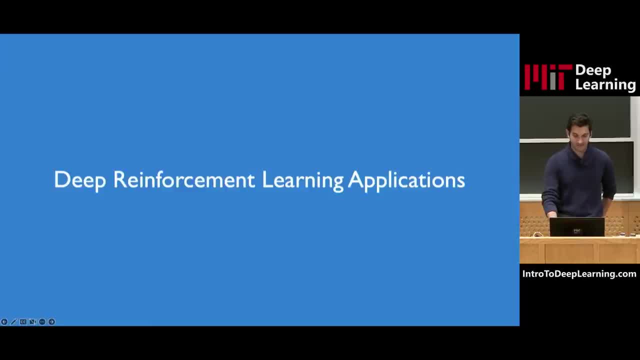 learning was used to train a policy end-to-end for an autonomous vehicle that could be deployed in reality. So that was something really cool that we created here at MIT. But now that we covered all of these foundations of reinforcement learning and policy learning, I want to touch on 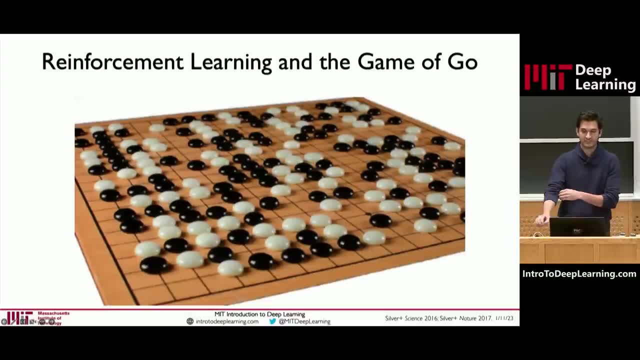 some other maybe very exciting applications that we're seeing, And one very popular application that I want to touch on is reinforcement learning, And it's a very popular application that I think a lot of people will tell you about and talk about is the game of Go. So here, reinforcement. 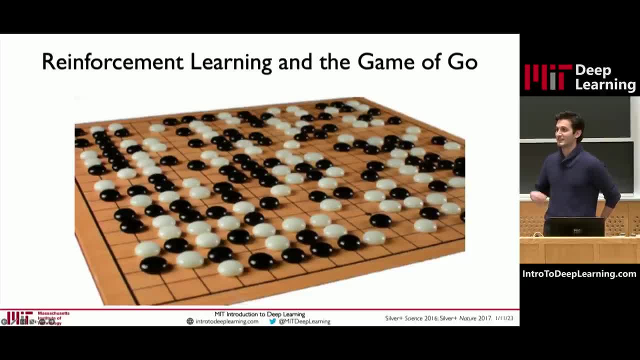 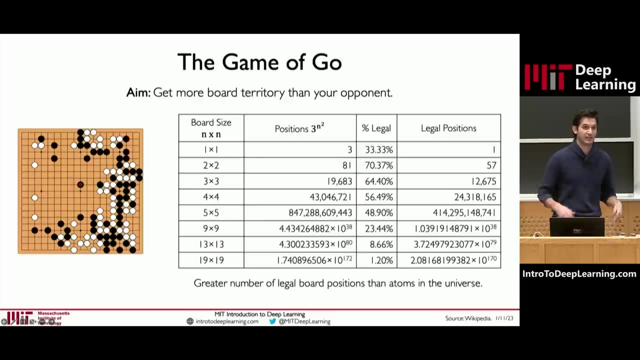 learning agents could be actually tried to put against the test, against grandmaster level Go players and at the time achieved incredibly impressive results. So for those of you who are not familiar with the game of Go, the game of Go is played on a 19 by 19 board. The rough objective. 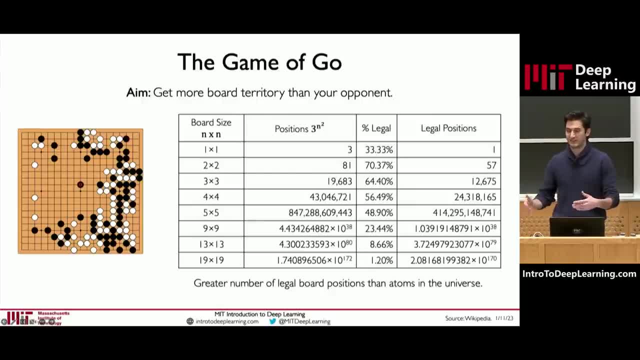 of Go is to claim, basically, more board pieces than your opponent And through the grid that you can see here, this 19 by 19 grid- and while the game itself, the logical rules are actually quite simple: the number of possible action spaces and possible states that 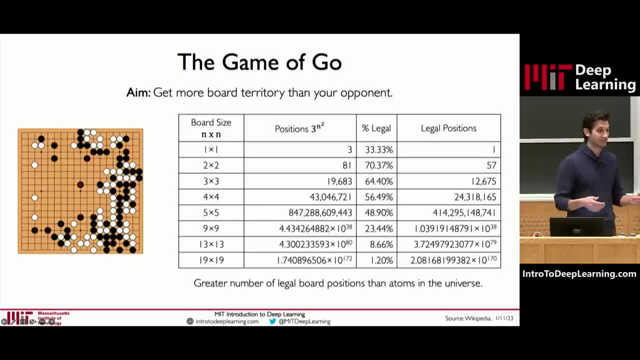 this board could be placed into is greater than the number of atoms in the universe. So this game, even though the rules are very simple in their logical definitions, is an extraordinarily complex game for an artificial intelligence. And so the game of Go is played on a 19 by 19 board, And so 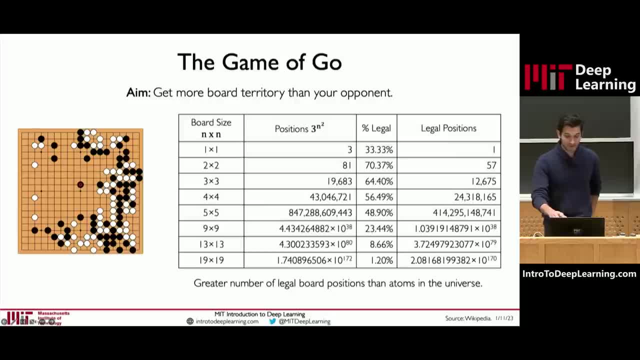 the game of Go's goal is to try and master the game of Go, So the objective here was to build a reinforcement learning algorithm to master the game of Go, not only beating, you know, these gold standard softwares, but also what was at the time, an amazing result was to beat the. 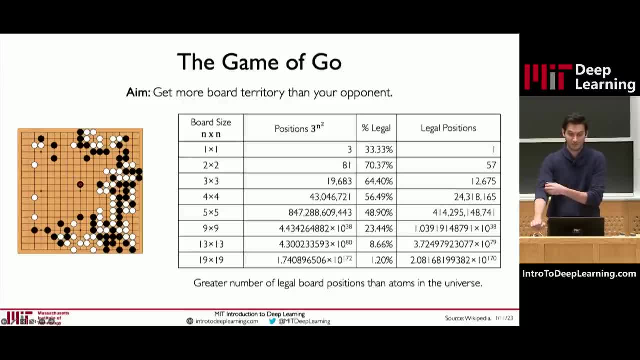 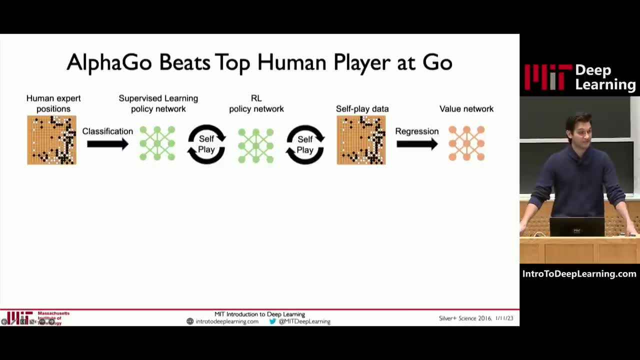 grandmaster level players, So the number one player in the world of Go was a human champion, obviously. So Google DeepMind rose to this challenge. They created, a couple years ago, this solution, which is very much based in the exact same algorithms that you learned about in. 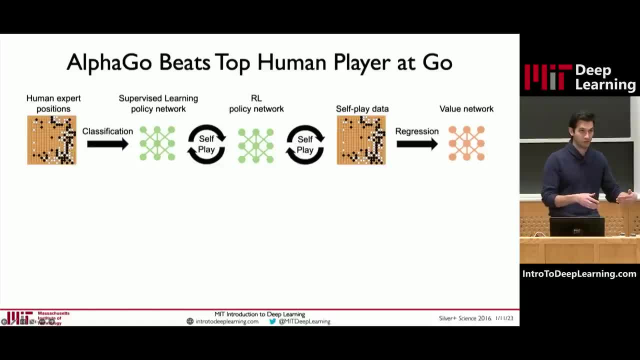 today's lecture. combining both the value part of this network with residual layers, which we'll cover in the next lecture tomorrow, And using reinforcement learning pipeline, they were able to defeat the grand champion, human players, And the idea at its core was actually very simple. 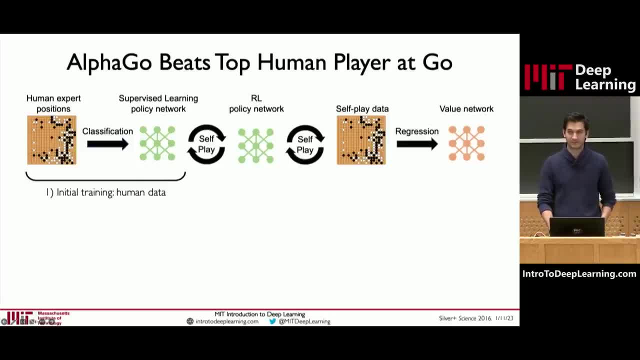 The first step is that you train a neural network to basically watch human level experts, right. So this is not using reinforcement learning. this is using supervised learning, using the techniques that we covered in lectures one, two and three, And from this first step the goal is to build: 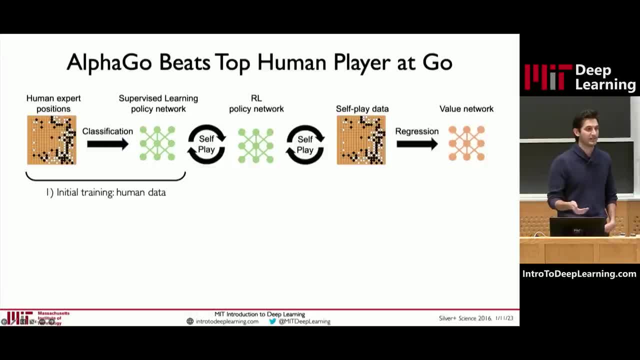 like a policy that would imitate some of the rough patterns that a human type of player or a human grandmaster would take, based on a given board state, the type of actions that they might execute, But then, given this pre-trained model, essentially, 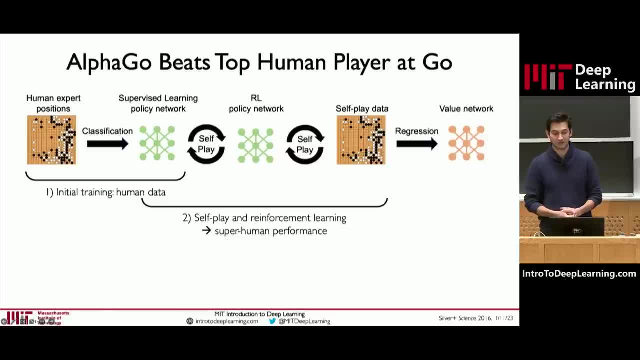 you could use it to bootstrap a reinforcement learning algorithm that would play against itself in order to learn how to improve even beyond the human levels. right, So it would take its human understandings. try to imitate the humans first of all, but then from that imitation. 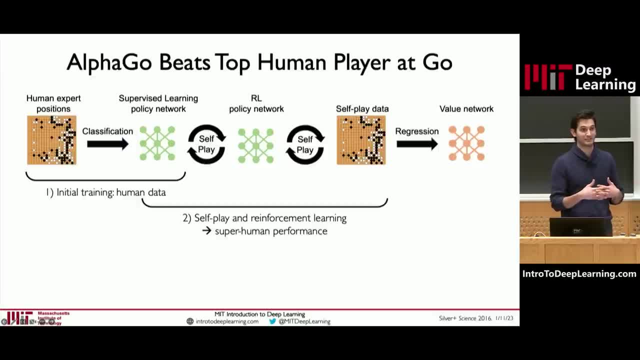 they would pin these two neural networks against themselves, play a game against themselves, and the winners would be receiving a reward. The losers would try to negate all of the actions that they may have acquired from their human counterparts And try to actually learn new types of rules and new types of actions. basically, that might be. 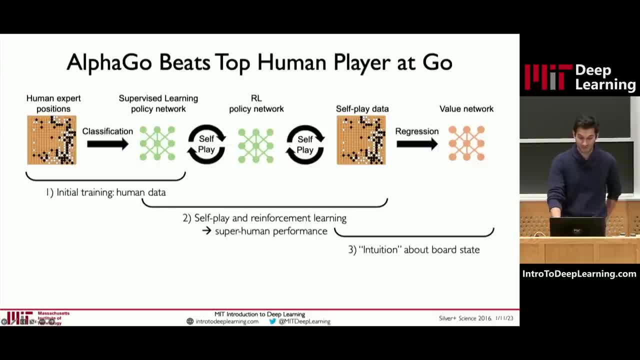 very beneficial to achieving superhuman performance, And one of the very important auxiliary tricks that brought this idea to be possible was the usage of this second network, this auxiliary network, which took as input the state of the board and tried to predict. you know what are all of the 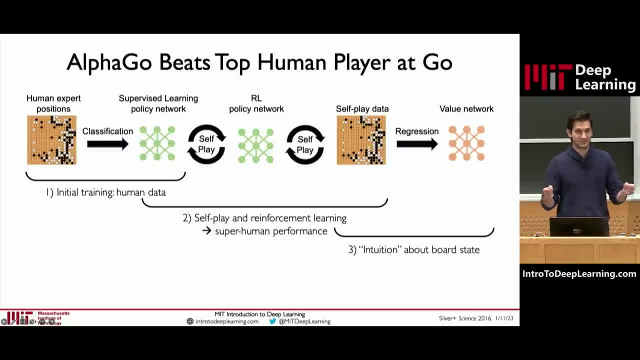 different possible board states that might emerge from this Particular state and what would their values be? What would their potential returns and their outcomes be? So this network was an auxiliary network that was almost hallucinating, right- Different board states that it could take from this particular state and using those predicted. 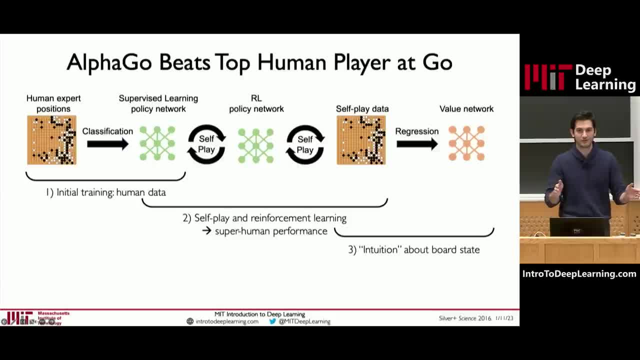 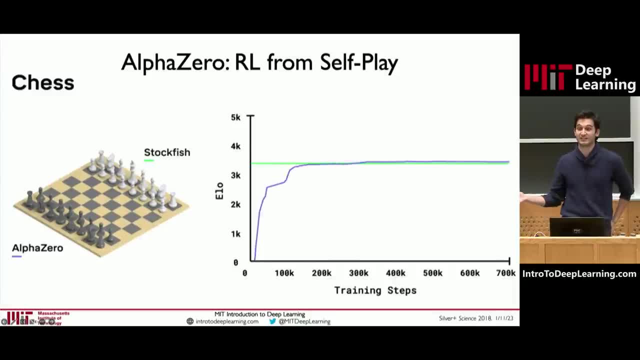 values to guide its planning of you know what action should it take into the future? And finally, very much more recently, they extended this algorithm and showed that they could not even use the human grandmasters in the beginning to imitate the human grandmasters. 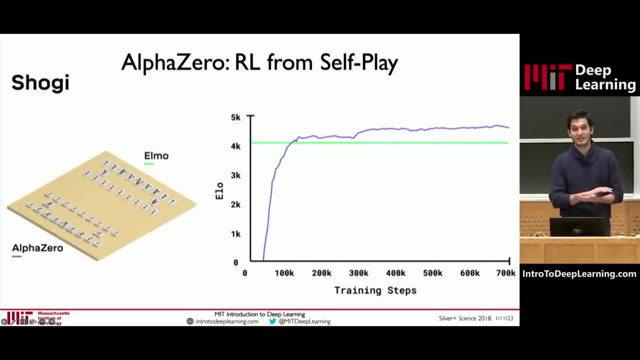 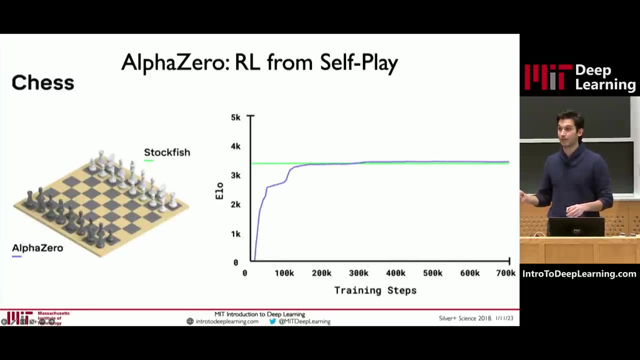 What if they just started entirely from scratch and just had two neural networks never trained before They started pinning themselves against each other and you could actually see that you could, without any human supervision at all, have a neural network. learn to, not only outperform. 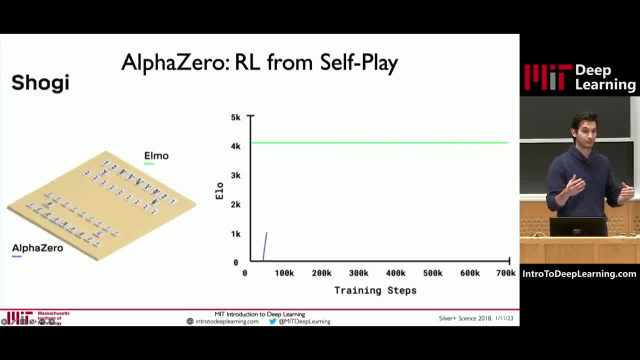 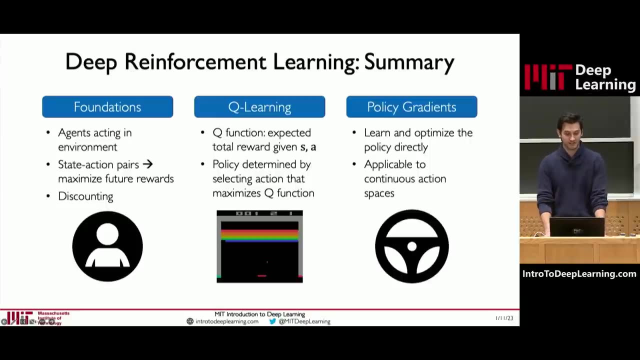 the solution that or outperform the humans, but also outperform the solution that was created, which was bootstrapped by humans as well. So with that, I'll summarize very quickly what we've learned today and conclude for the day. So we've talked a lot about, really, the foundational algorithms underlying reinforcement. 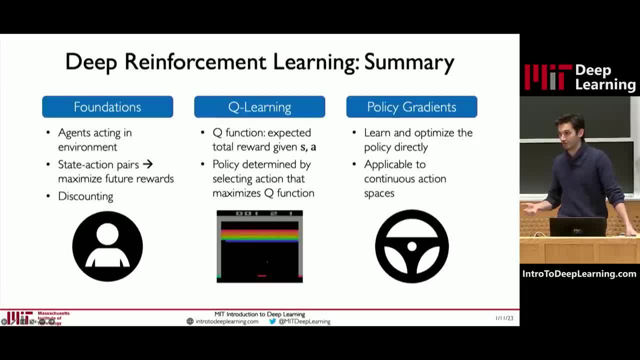 learning. We saw two different types of reinforcement learning approaches of how we could optimize these solutions, First being Q-learning, where we're trying to actually estimate, given a state, you know, what is the value that we might expect for any possible action. 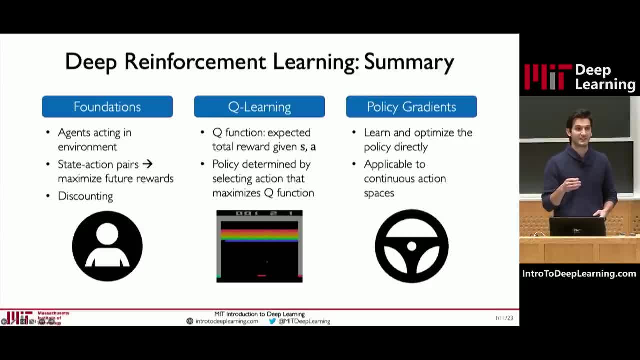 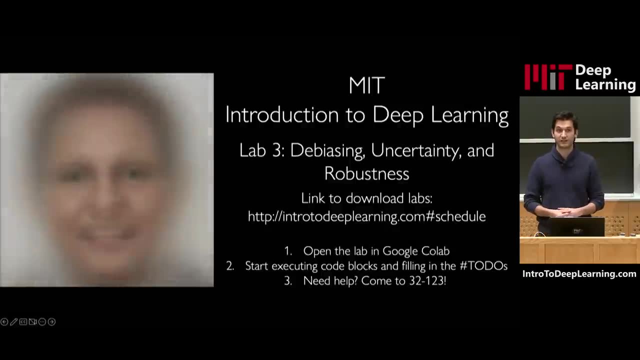 And the second way was to take a much more end-to-end approach and say how, given a state that we're in, what is the likelihood that I should take any given action to maximize the potential that I have in this particular state? And I hope that all of this was very exciting to you. Today we have a very exciting lab. 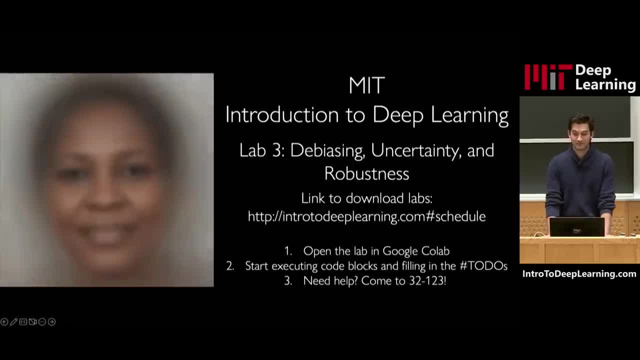 and kickoff for the competition And the deadline for these competitions will be. well, it was originally set to be Thursday, which is tomorrow, at 11 pm. Thank you.